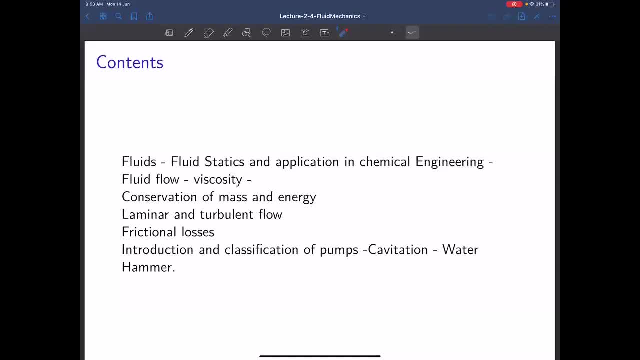 we are using it, we are going to use it also. and laminar and turbulent flow, also today you'll see- and followed by frictional losses and pumps. so, to the extent possible, we'll see at least. yeah, these two we'll see today and the other two, uh, we'll see in the coming classes. so by 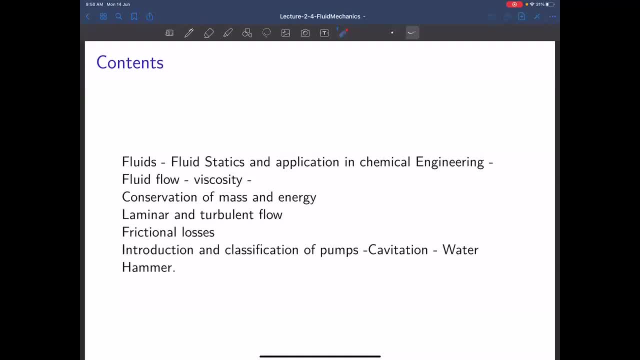 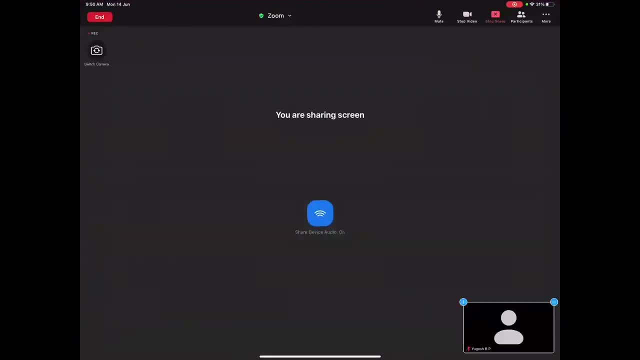 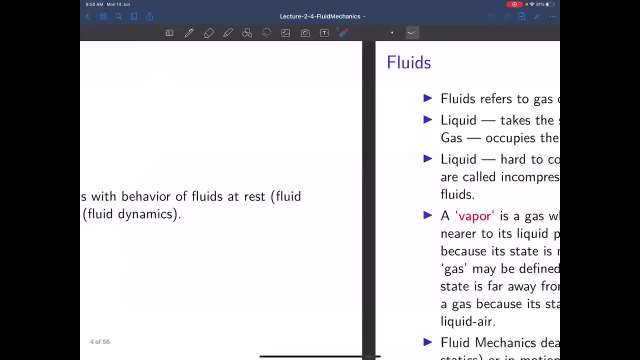 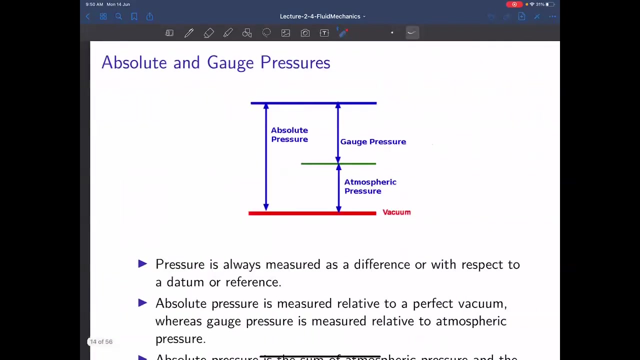 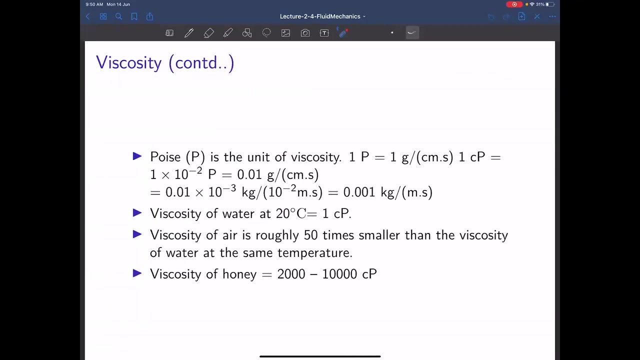 this weekend we'll be done with this, uh, plate mechanics chapter. so how many are available? let me see about 48, 47. fine, good number back to my screen, okay. uh, fleet static, fleet dynamics, these are all known to you, fine, uh, the unit of viscosity is centipoise one. one price is one gram per centimeter second. 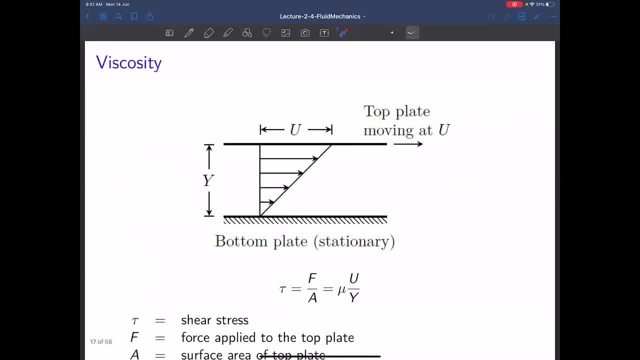 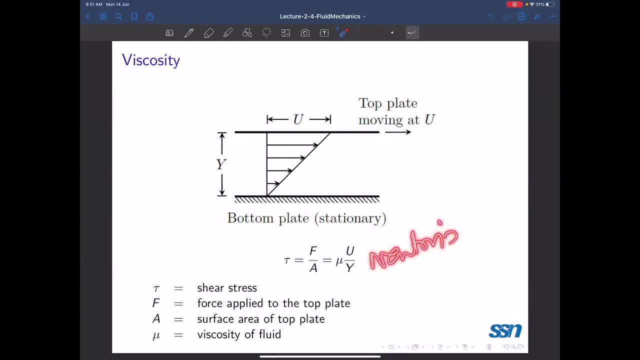 why this is coming. these are all coming from your, uh, this equation, what is called as newton's law of viscosity. uh, of course. uh, not all the fluids obey this very simple relation. they also have some other dependency. uh, otherwise, the fluids which obey this newton's law of viscosity, all are called. 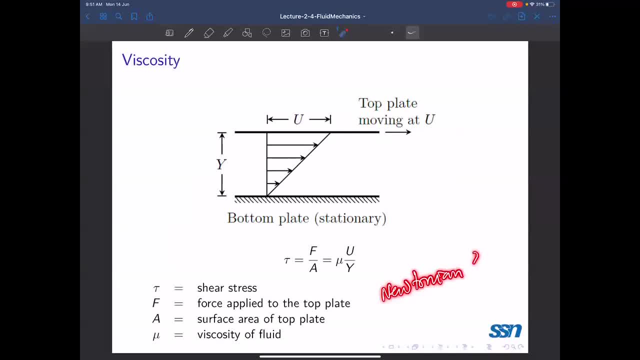 as newtonian fluids. okay, this thing i haven't written in the slide, otherwise i can know down this: the fluids which follow this newton's law of viscosity are called as newtonian fluid and which don't follow this they are called as non-newtonian. uh, of course water is a nice. 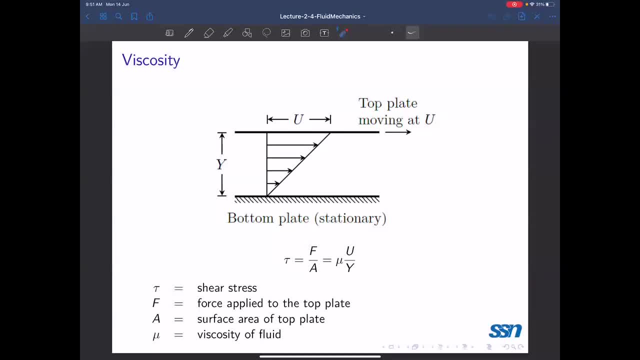 example for newtonian fluid water. yeah, these are all the nice examples for newtonian fluid uh. for non-newtonian we can give examples like our: uh, even the honey is also non-newtonian. and not only that, the glycerin solutions and 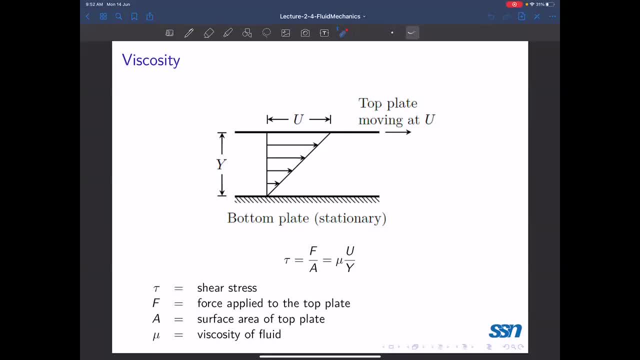 i'm not sure about glycerin. this honey is kind of the non-newtonian and even the toothpaste. whatever we have, this toothpaste we apply regularly. uh, this toothpaste is also a kind of fluid. initially it's appeared to be a solid and if you apply, 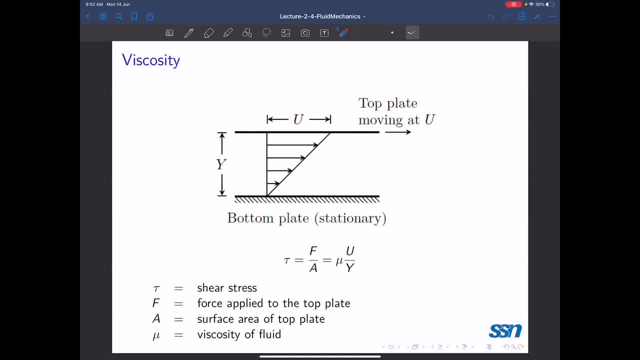 uh, force, uh, what is called as a shearing force. now, on the tube side, we'll apply a shear force. it tends to flow out from the mouth and you are seeing that and again it is uh sticking. otherwise, whenever you apply certain extra force, it is flowing. otherwise, they uh don't initially start. 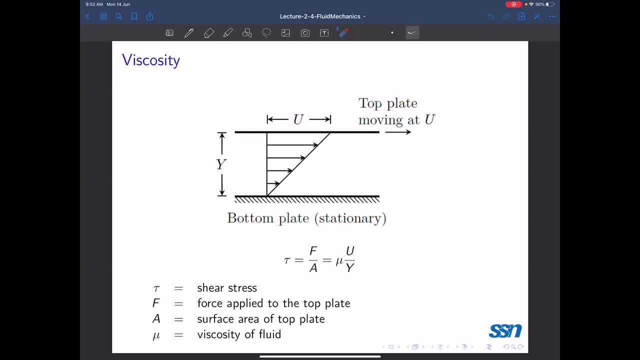 to flow after it. uh, it flow after certain application of uh, otherwise, uh, once uh stress is exceeding a minimum stress. otherwise, if you want to write the equation of the flow of the solution for such a fluid, you need to write this: tau plus tau not equal to, otherwise tau equal to. 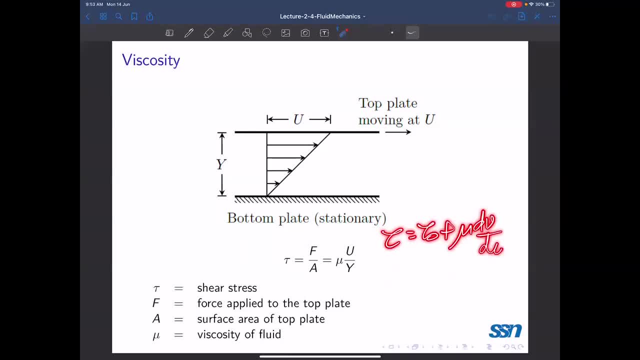 tau naught plus mu into dv by dy. so this is the case with this fluid, which is what is called a toothpaste. otherwise, we'll uh name that fluid as what is called bingo plastic. no need to worry about this terminology, we are going to study them in your fleet mechanics course. okay, i need not want. 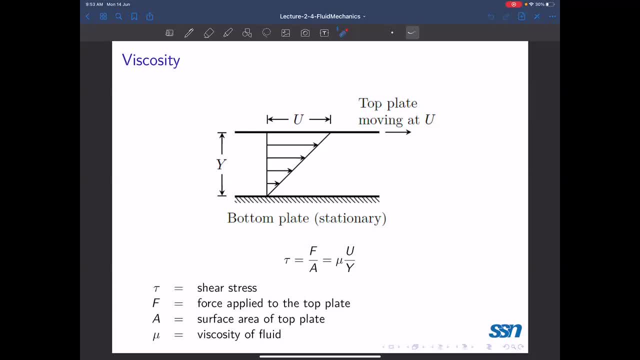 to load you with much terminology. okay, this shear stress is about the force, shear force. shear force means the flow of force. obviously you have a plate like this and here in the bottom you have a plate and the top plate is moved. uh, the bottom plate is held stationary and the force required to move the top plate 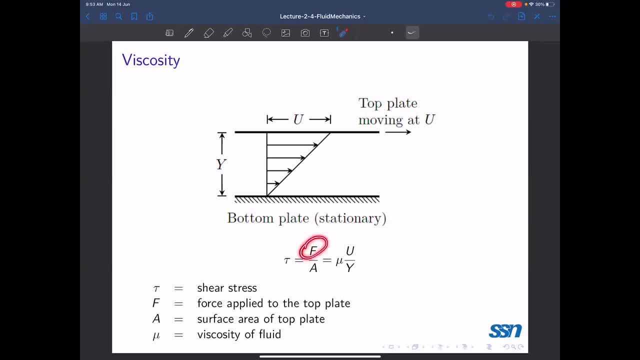 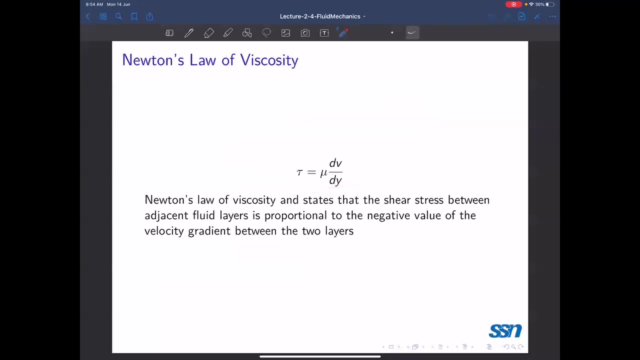 and a velocity v is given by the shear force, uh, the area of plate in contact with the plate. that is a year. so this force by area, shear stress, uh, which depends on the uh velocity gradient, or is the velocity divided by the distance velocity gradient? okay, so newton's law of viscosity? uh, okay, this already we have. 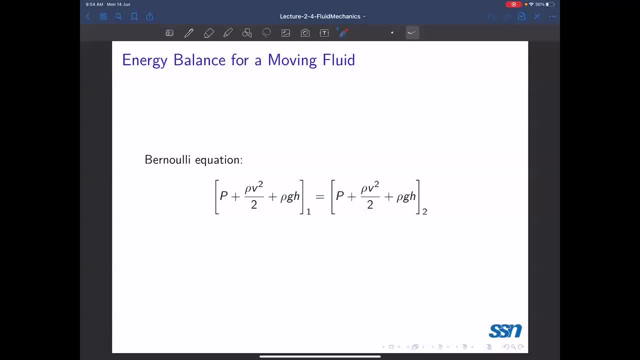 given, and okay, then today's class, we are going to see the application of this uh bernoulli equation for flow measurement. in the last class we have, i have indicated this, uh, how this is used for. uh, this, what is it? uh, a carburetor, uh, uh, a carburetor, uh a carburetor. 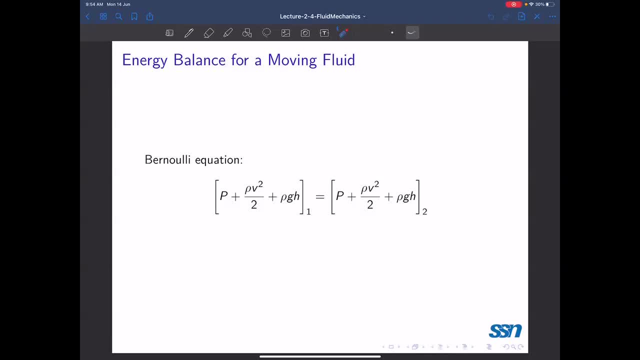 is used for energy. uh, this how to how it is used for taking the fuel to the carburetor or engine through the carburetor. okay, that i will see that, so that uh, i always this. uh every thing is uh in pressure time. uh, every terminology is having units of uh newton, per. 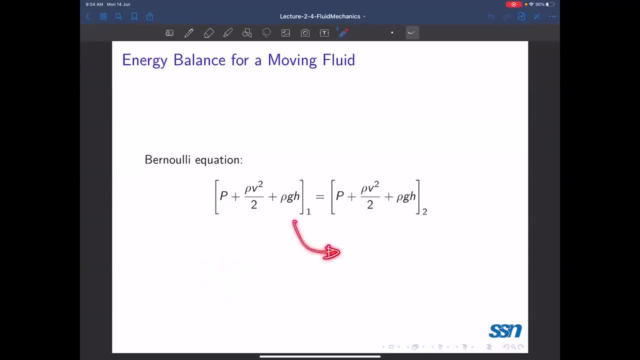 meter square p is in newton per meter square. this you can ensure that you can check. this rho gh- multiplication of rho gh is also in newton per meter square. this rho v square by 2 is also in newton per meter square. can we, if you want, you can verify. this row is in. 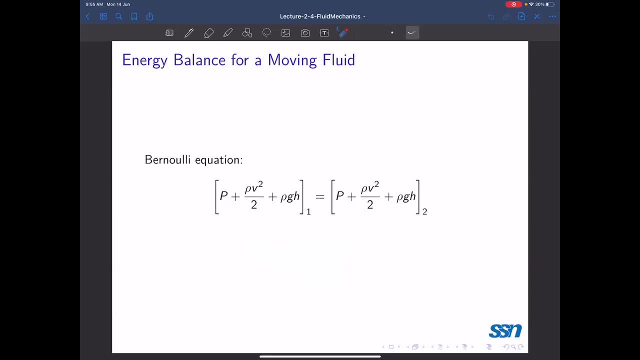 kg per meter cube and v square is in meter per second that whole square. you check whether the unit is coming to that of newton per meter square. what is newton? this is kg into meter per second square divided by meter square. so this you can check, check every. everything is having the same. 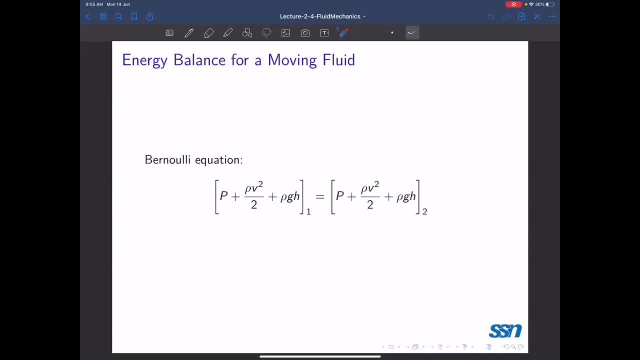 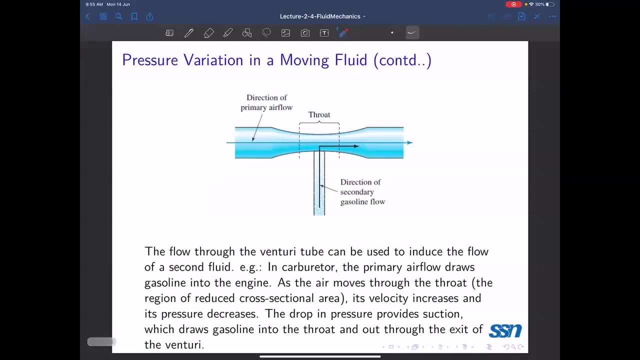 units, then only you can add the terms. otherwise, uh, dimensional consistency would be there whenever you add any terms. okay, okay, this carburetor, uh the- yeah, of course- air is uh taken into the engine and along with that, fuel is also sucked into the engine, uh, through this part of the throat. 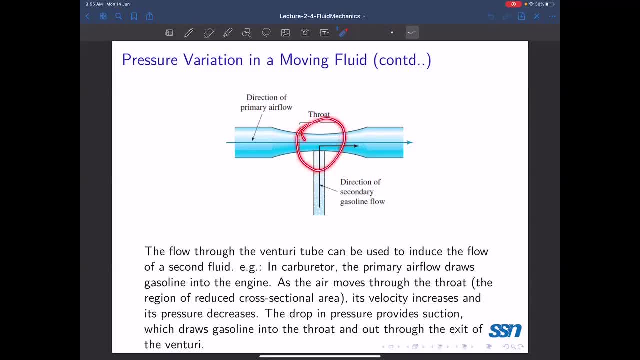 this is because of a low pressure created in this area. the low pressure is created because of there is a reduction in area. the reduction in area leads to increasing the velocity. so increase of velocity leads to decrease of pressure because, uh, both are the same potential levels. so we have p1 by rho g. 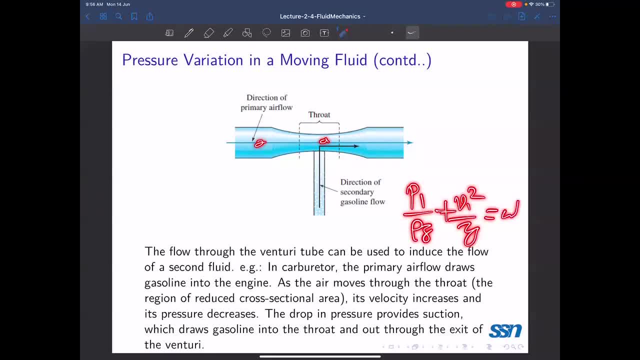 plus v1 square by 2g, that is equal to constant uh. so otherwise, whenever the pressure decreases, of course velocity increases because of the reduction area. so whenever the velocity increases there is associated drop in pressure. so this area is in low pressure, so the fuel in the tank is automatically. 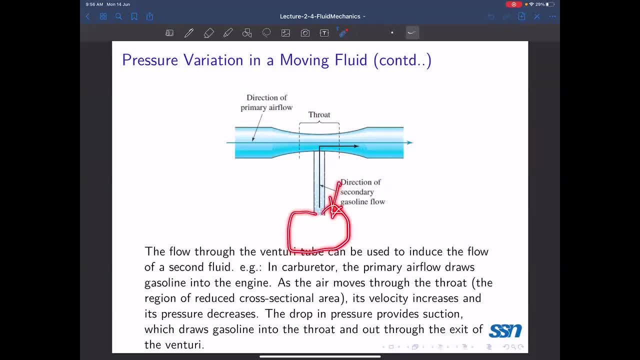 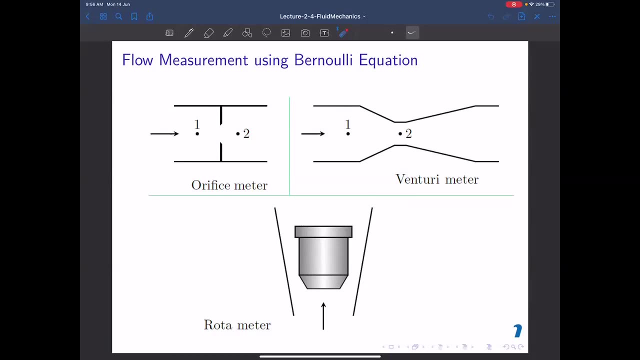 taken in because the fuel tank is in atmospheric pressure. so here you have a low pressure, so it is taken in. uh to the uh. what is that device? okay, that we are going to employ this, uh- bernoulli principle for flow measurements? okay, the understand- i will come to this later- what is called zero two? 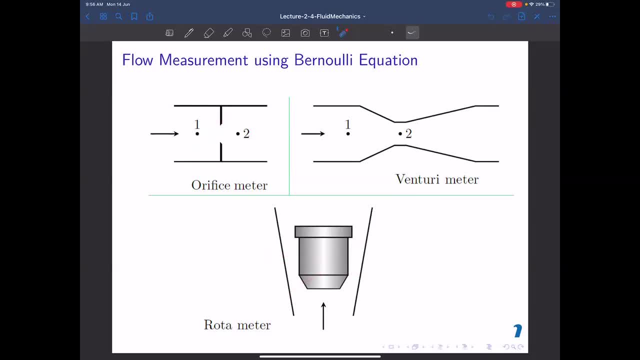 rotameter see uh. even this also we'll see later. this is the same device as we have used for carburetor. you know what is a venturi meter. we are going to use this for uh flow measurement. uh, we know already. we know the device, the pressure for pressure measurement we can. 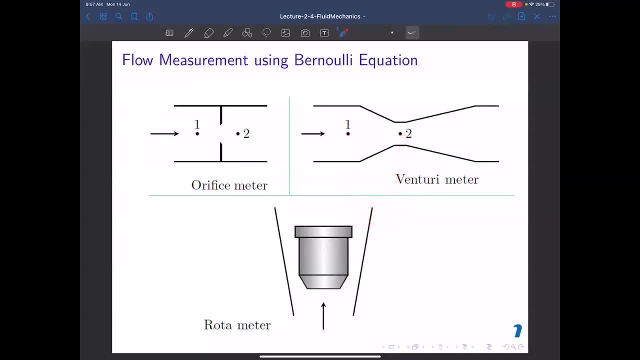 employ a nanometer, otherwise we can connect a nanometer to measure the pressure difference between point one and two. uh, uh, otherwise we are going to create a pressure difference by, by making a reduction in area. so we are. so there is a pipeline, we are suddenly reducing the cross. 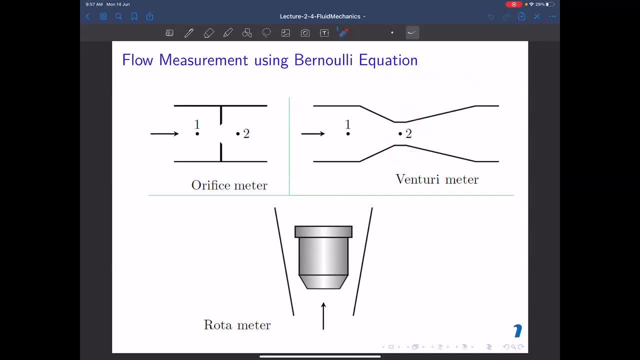 section and, uh, creating a increase in velocity. so in comparison to velocity at section one, velocity of section two is more because area is lesser. yeah, so because a1, v1, there is a volumetric flow rate in equal to a2, v2. so since a2 is lesser, v2 has to be higher. okay, so always v2 will be higher than v1. 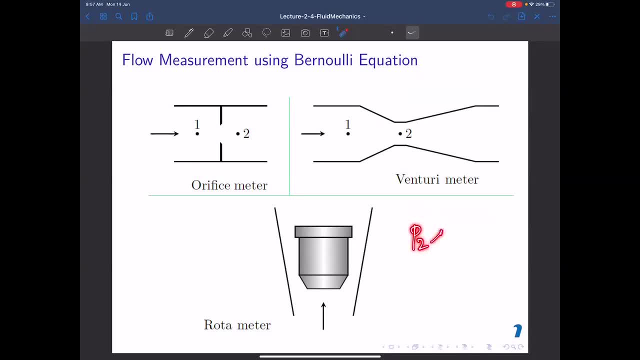 since v2 is higher than v1, uh, p2 will be lesser than p1, so, uh, there will be a pressure difference created. this pressure difference is in proportion to the velocity difference. okay, i, i can write here, you can write this, and we can make a derivation of this matter. let me take a nice 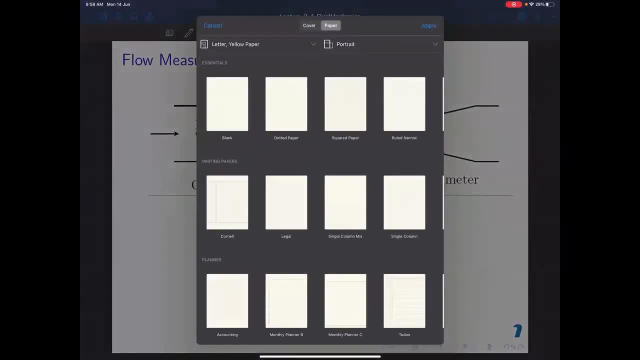 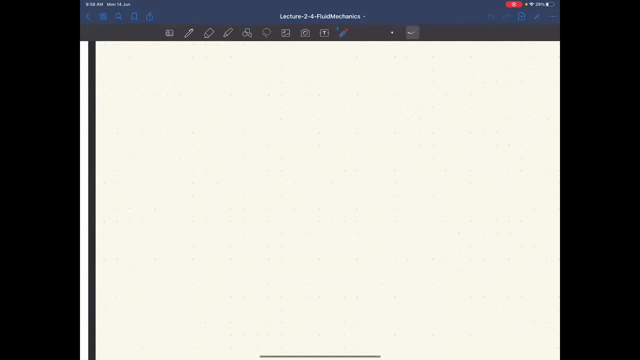 template is. I am going to develop this equation to measure the free flow so that this derivation is simple, only so. that's why I am trying showing this. maybe you would have come across this answer, I don't know. so we have this pipeline, we are making a reduction in. 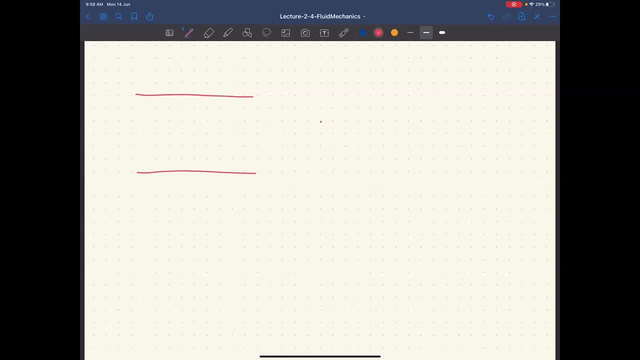 cross section. let us take the points in points. okay, uh, there is a small reduction in cross section and again bring it to the same cross sectional area. till this point, yeah, right, yeah, the start and paper is nice now at least. so, uh, sorry, uh, it should have been stopped at this point. 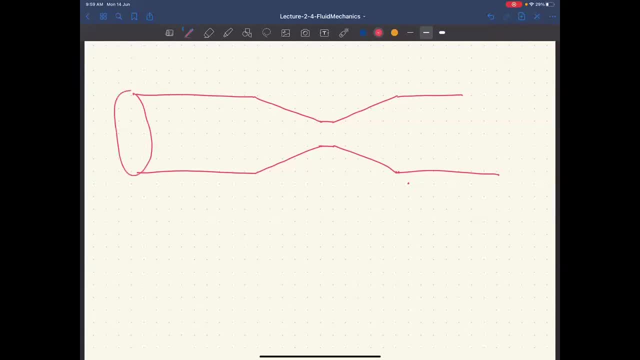 okay, uh, of course, this is a cylindrical pipe now, so we have, we are going to make a pressure measurement. this is your section one. this is section two. to these, between these two points, let us connect a manometer. the simplest manometer is u-tube manometer. already, you know how to draw a manometer. okay, nice u. 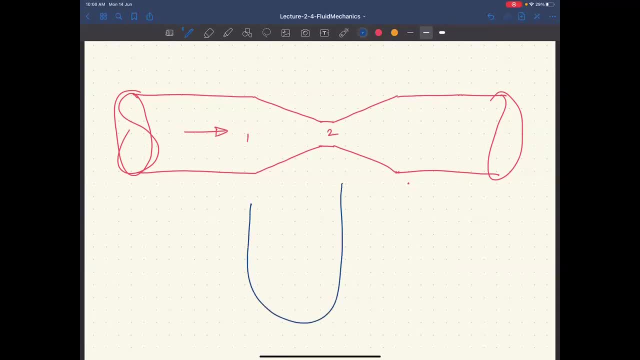 nice u-tube manometer connect these. of course it's a cylindrical tube. yeah, draw with uniform procession. okay, uh, i could not draw that nicely. okay, uh, this is connected here and this is connected to this point. okay, so let us draw some manometric fluid. uh, naturally fluid uh, at one is at high pressure and fluid two is at low pressure. how do we say? 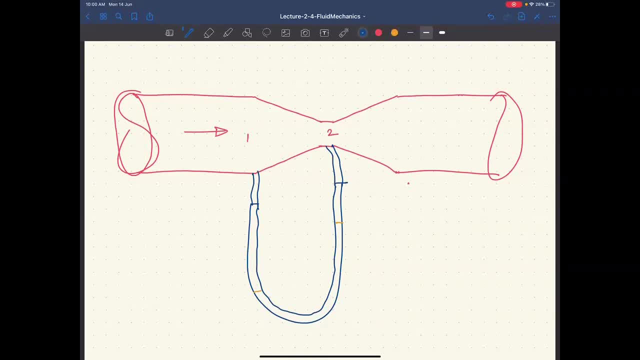 again. let us write this bernoulli equation, bernoulli equation, bernoulli equation. this Bernoulli equation is: p 1 by rho, g plus v 1, square by 2, g plus h 1, equal to the same way, I think, with 2 and again h 1. we need not do this because level at 1 and 2 are nearly. 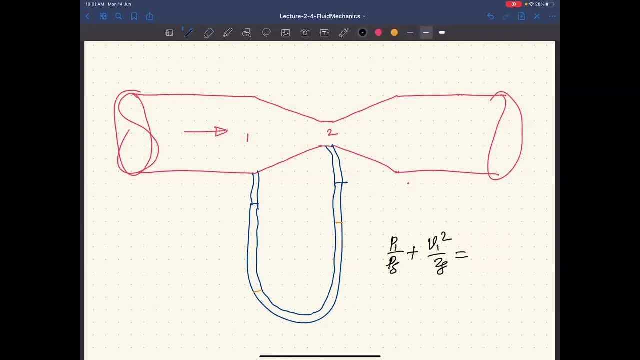 the same are the same. otherwise we can simply deal with pressure and pressure, energy and pressure and velocity terms alone. So we have p 1 by rho g, p 2 by rho g plus v 2 square by 2 g. So otherwise we have created a pressure difference between 1 and 2. otherwise p 1 is 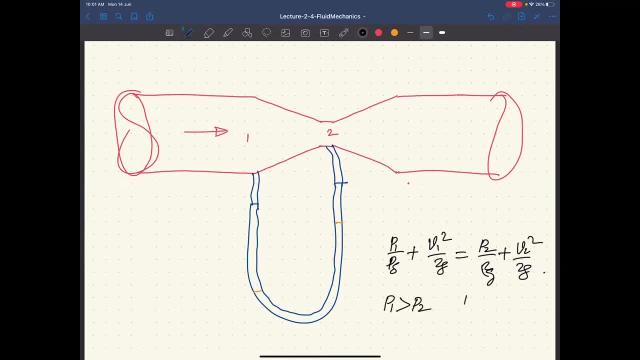 higher than p 2. how do we say this? because v 2 is higher than v 1. since v 2 is higher than v 1, p 2 is lesser than p 1. that is in that way you can argue. So v 2 is higher. 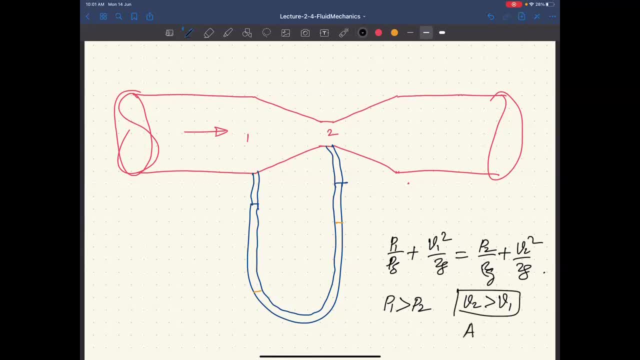 because this is from mass balance, from mass balance. So these are volume balance. volume balance you can easily apply for liquids, but mass balance is the very common thing. So a 1 v 1 equal to a 2 v 2, of course, to be correct. 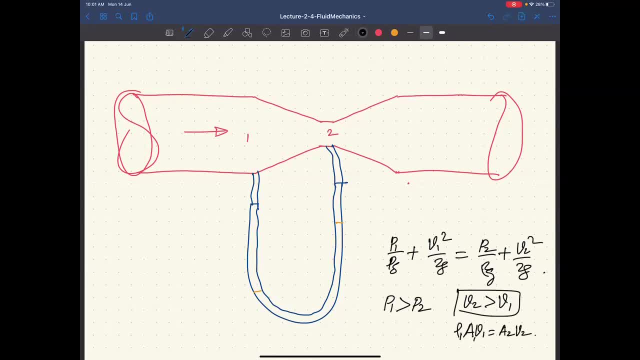 you want to, you should write it as: rho 1 a 1 equal to rho 2 a 2 v 2, since rho 1 and rho 2 are nearly are the same. otherwise for liquids the density difference is not much because of any appreciable change in pressure, So otherwise they are incompressible fluid. So 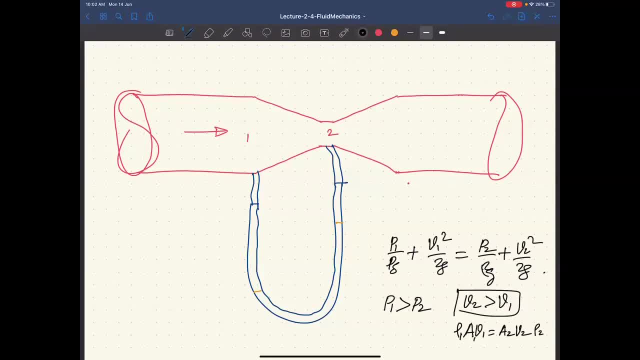 a 1, v 1 equal to a 2, v 2. otherwise, simply, v 2 is higher than v. 2 is equal to what is it? a 1 by a 2 into v 1.. So naturally, this a 1 is higher than a 2. what is a 1 and a 2? 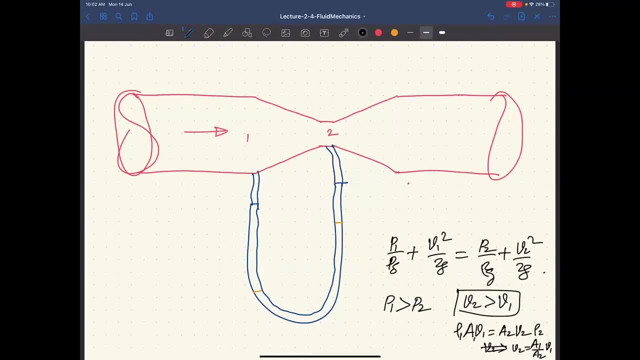 are. a 1 refers to the cross sectional. what is it? the pipe cross sectional area at point at section 1.. So section 1 is here and section 2 is here. So definitely v 2 is higher than v 1, ok, and 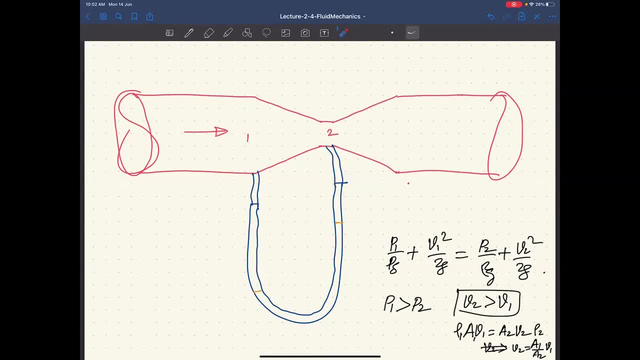 because of that, p 1 is higher than p 2. this is from coming from this Bernoulli equation. So the what is the manometric fluid available here? this is where manometric fluid, So manometric fluid, manometric is, manometric is, manometric is giving, manometric is giving a level difference. 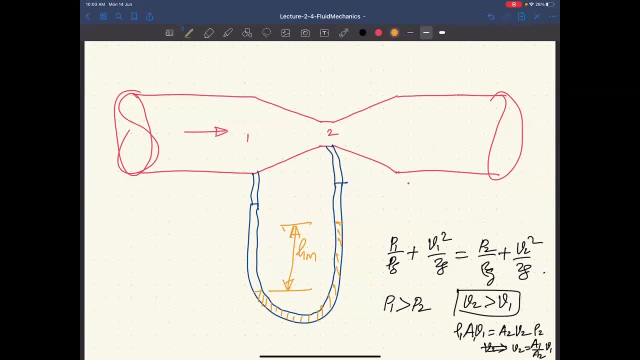 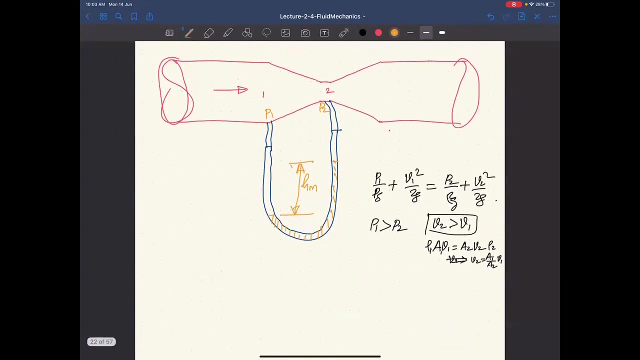 of of hacha. ok, So this is where p 1 and p 2, ok, fine. So what is our ultimate thing? we want to find the velocity at point using this manometer level difference. ok, let us take one more sheet. fine, 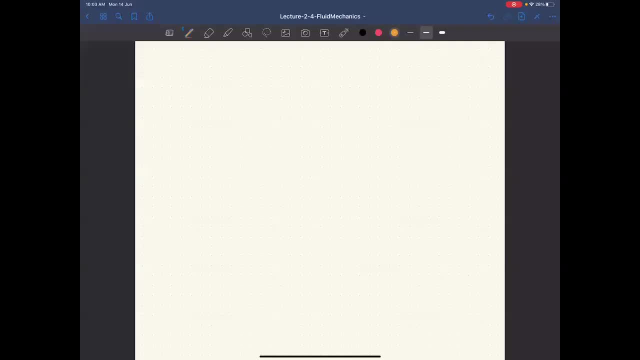 So v1 square by 2 g. okay, so since everywhere g is there, we can remove that and we can write this: 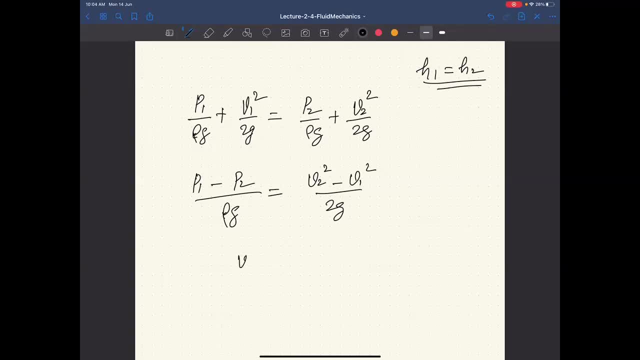 and again. okay, one minute clear, so we can write this: v1 in terms of v2. how do you write v1 in terms of v2? a1, v1 equal to a2, v2, so v1 is equal to a2 by a1 into v2 and since area is proportional to d square, what do? 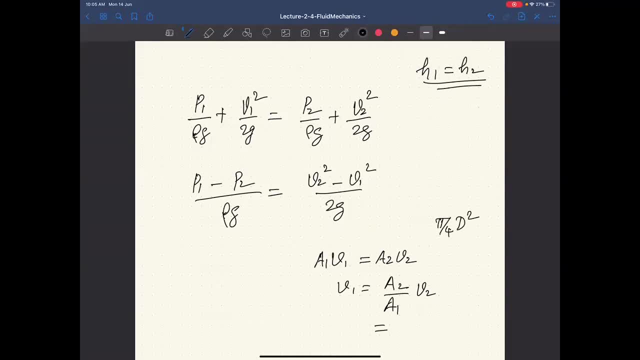 you say area equal to pi by 4 d square. so so this is a flow cross area. so a2 by a1 is simply equal to d2 by d1 square, or is d2 square by d1 square into v2, so otherwise you can replace this v2. 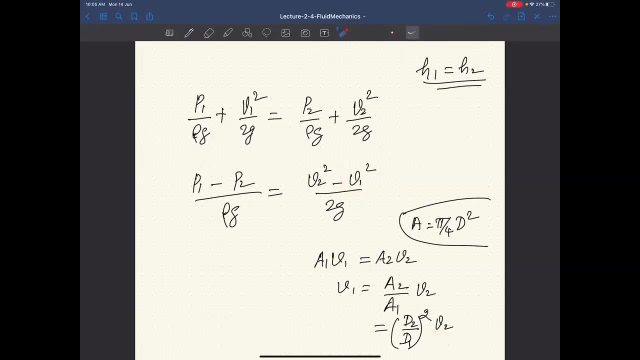 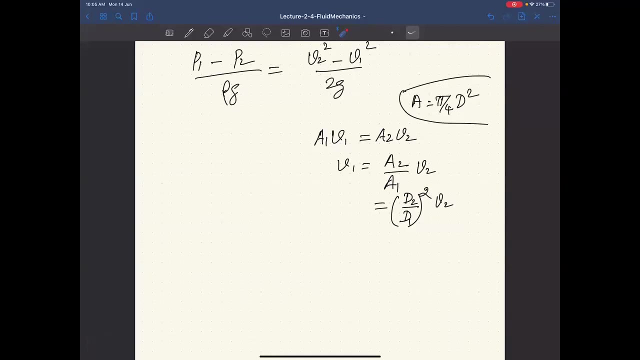 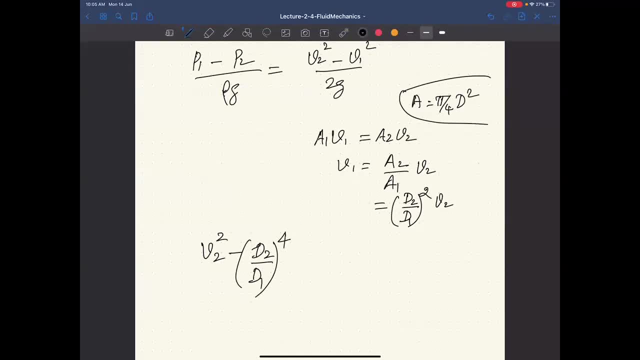 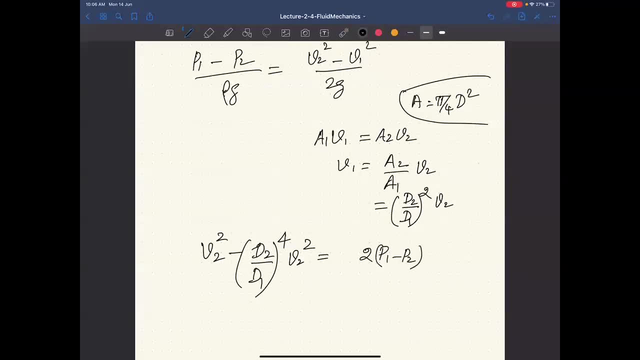 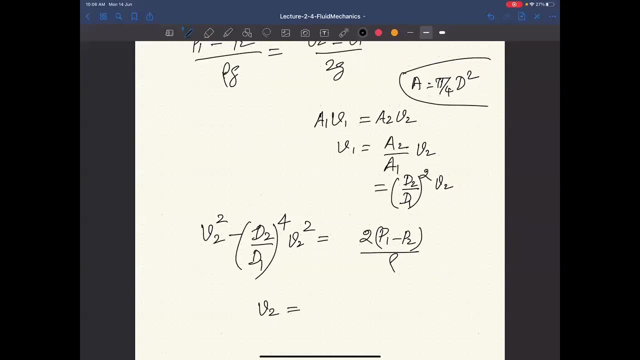 two into p1 minus p2 right and the row sorry, yeah, fine, ah, this again you can rearrange. so always we will write this v2 as root of u into p1 minus p2 by rho into 1 by 1 by 1 minus V 2 by V 1 to the power 4.. Again, it will be square root. 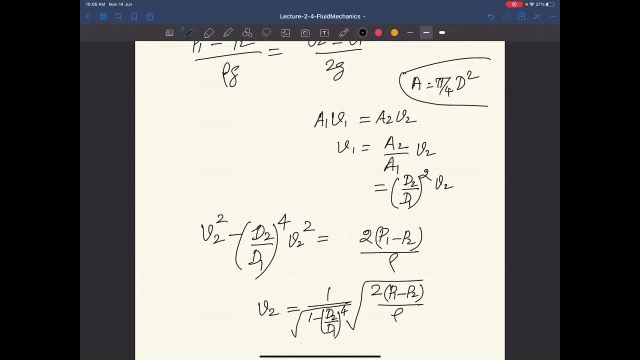 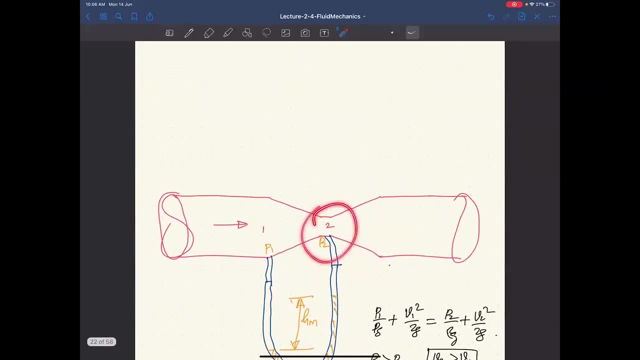 here Fine? no, Because V 2 square is having this terms: 1 minus V 2 by V 1 power 4.. So R is V 2, is this? So this is the expression for velocity of fluid in the this reduced. 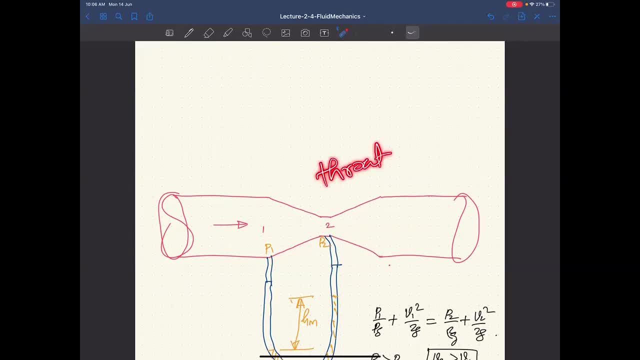 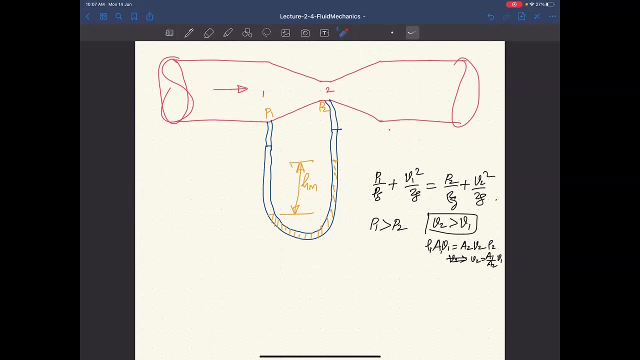 cross section, what is called as the throat section, Throat section R is that we are creating a reduction in area, thereby creating a pressure difference, And this pressure difference is measured with a device, say, simply by nanometer or any other pressure measuring device. So 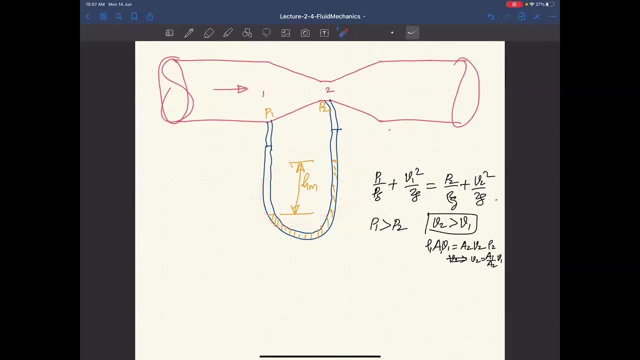 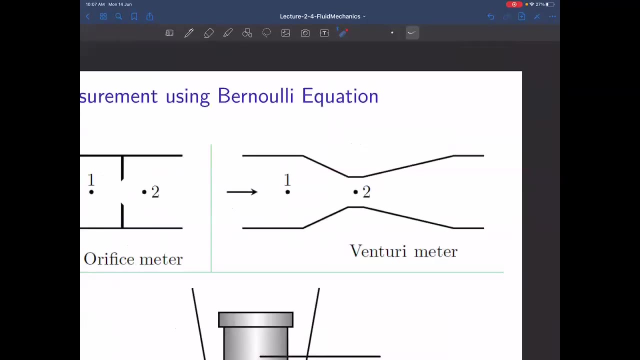 this measurement of pressure difference is giving you indication of velocity of the fluid in this area. Of course, if you know the velocity in this area, you can also say about the velocity in this section, Because area relations are known to you. So using that, you can see. This is what is the derivation. 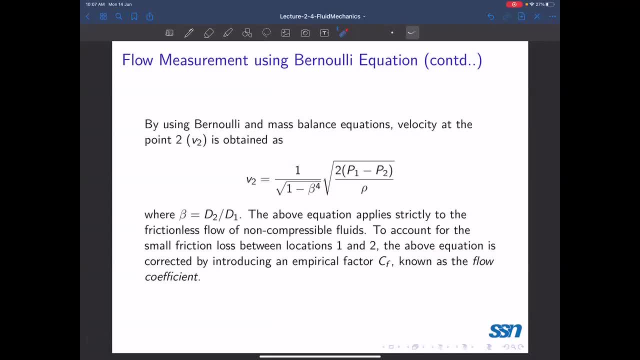 So this derivation you can make and you can get the velocity of the fluid in the point 2.. The same way you can also get the velocity at, So so you can get the velocity at any other cross section. Otherwise, this is this equation. 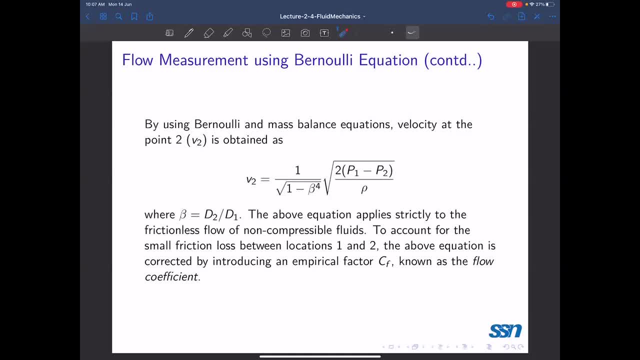 is coming simply from the application of Bernoulli equation. Always, if you look closely at the equation, what is that? simply V equal to root of root, 2, g, h, this, what is this? delta p by rho? This is p 1 minus p 2 by rho. delta p by rho. We know this. delta p by rho can be. 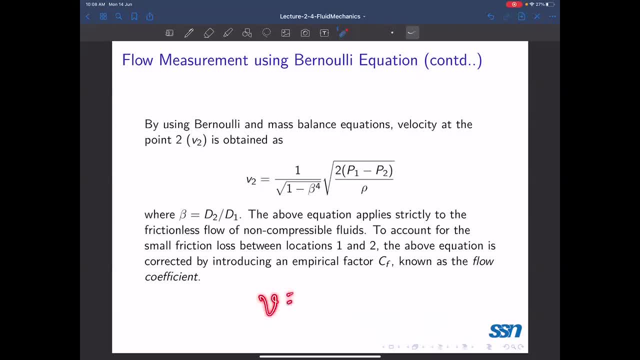 also equal to g h. So we are going to use delta p by rho whole. So we are going to use delta p by rho whole. is b equal to simply coming as g? h, except for the smaller terms like 1 by 1 minus p? 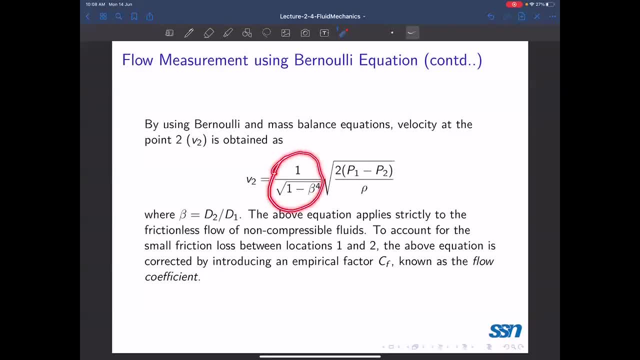 top over 4. this is to account for the change in the area we have already come across with this equation in your physics itself. what is that? the equation even i have, even last class also. you have some, some of you have also said about this equation: uh, for finding the 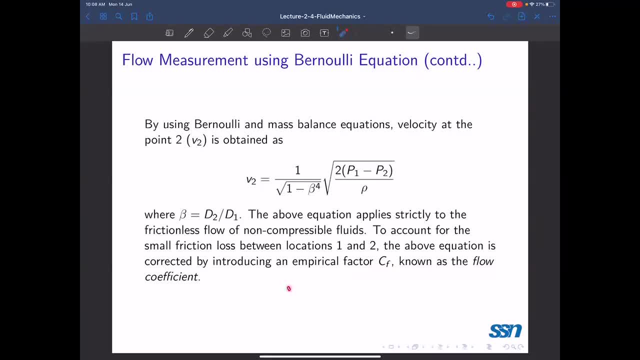 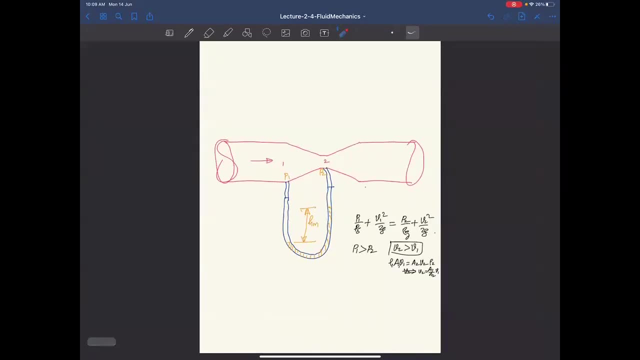 velocity of the free zeta. yeah, right, uh, otherwise, what is called a star is the equation. okay, so otherwise, uh, this bernoulli equation, uh, using bernoulli equation, you can measure flow in a pipeline. uh, easily, or simply by connecting a pressure cage between these two points. 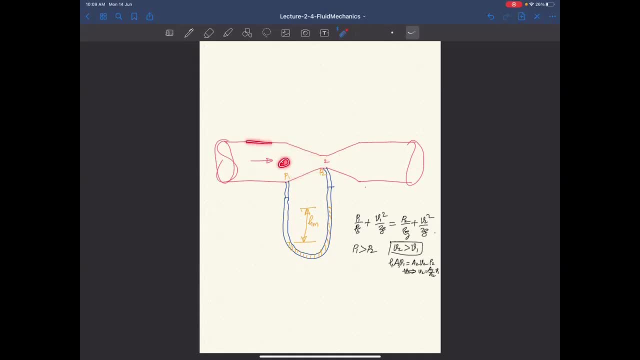 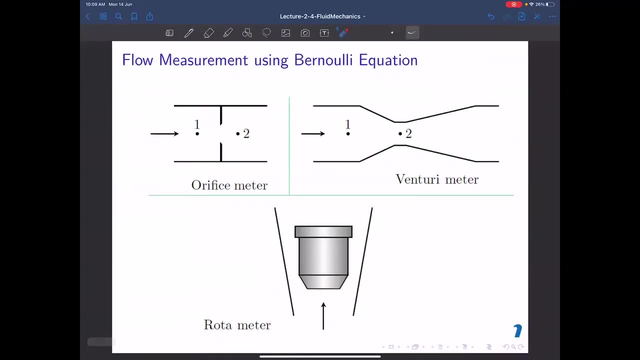 of course these party. two points means. the one point is of the rapid cross section, another is of reduced process. in the same way we can also uh, create a, otherwise we can make another kind of device. this is an entry meter- is having a nice reduction in area, whereas the another device, what is called as orifice meter, 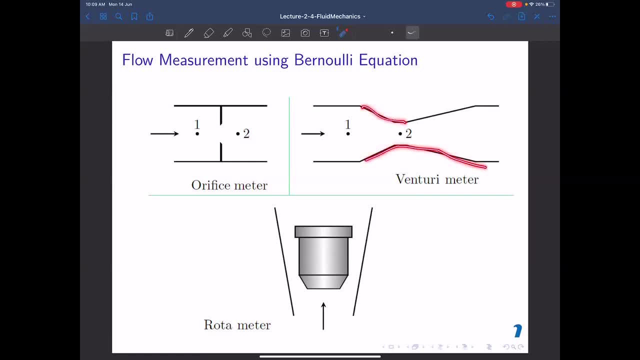 we don't have such a reduced, smoothly profiled flow we have always. we simply put a plate in the flow, uh, because of which the flow has to make a like this: they have to pass through this uh throat section, otherwise they will diverge. sorry, convergent again, it will diverge. 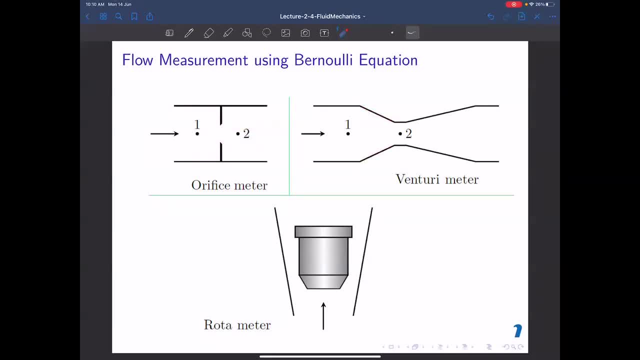 otherwise. this is here: there is a smooth flow, whereas the fluid has to make a sudden change in area and again, uh, diverge otherwise. this rvs matrix is simple in construction. uh, i will simply put a plate in the receive a pipeline, simply cut the pipeline and 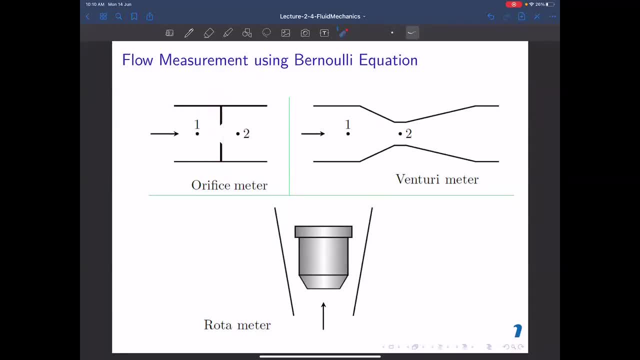 connect this disc and connect the disk and measure the pressure difference between this inlet and outlet. this point two is nothing but the point of, uh, convergence. the fluid is converging and again making it diverging, otherwise, if you see the flow, so it will actually try to converge and again only diverge. 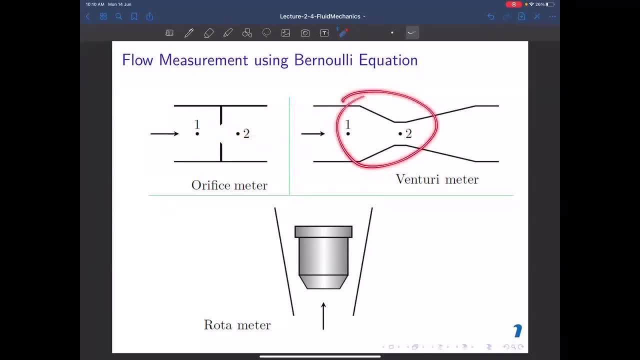 all right, here we are making such a cross section and by this mechanical means here we don't make such a this shape simply by putting a disk plate and creating a pressure difference. this pressure difference between one and two can be measured as like here, and the same equation is applicable here as well. uh, but if you compare these two meters, 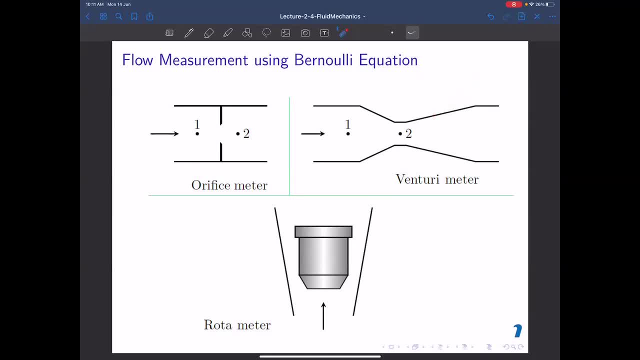 this venturi matrix uh venture meter. you need to have additional uh this kind of section, whereas here only one plate is enough. uh. but if you compare the present or with the frictional losses, that means there is a loss of energy in the form of friction that we are going to. 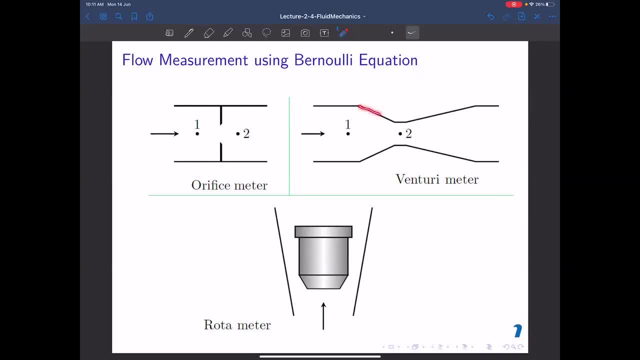 again correlate. let's see, uh, since we are reducing the cross-section smoothly and again expanding it smoothly, uh, the energy loss in the form of friction is actually minimum in this venturi meter, whereas here in this orifice meter, uh, suddenly the fluid has to reduce in cross. 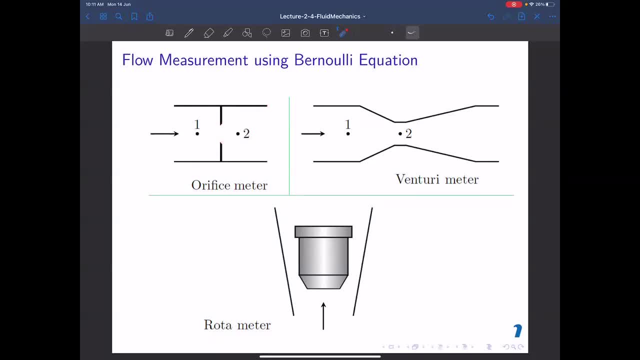 section and again they have to convert diverge service. there are a lot of losses in this section of this pipeline. so otherwise this orifice meter is simple in construction but it is creating what is called permanent energy loss to the fluid. okay, all you will study in your rough read mechanics course in very detail. at least you should know now. 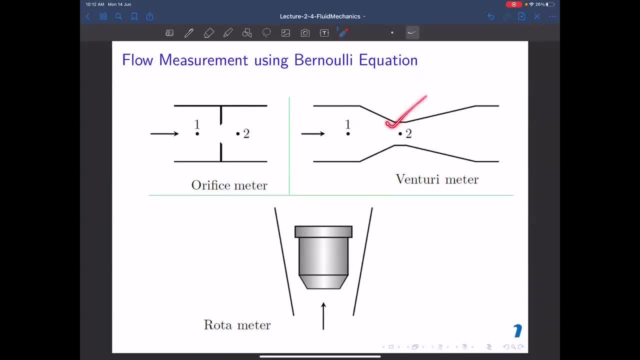 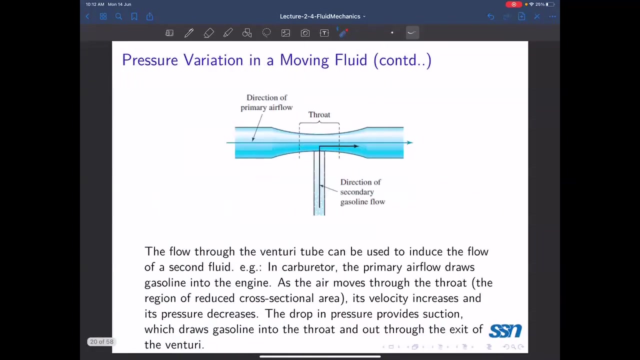 uh, this kind of devices- venturi meter and orifice meter, these are all available for flow measurement. uh, simply, they are utilizing the principle of bernoulli equation to create a reduction in cross-section and they will create a pressure difference and measure the pressure difference. uh, and that is uh giving you the idea of the velocity uh, in the pipeline. okay, 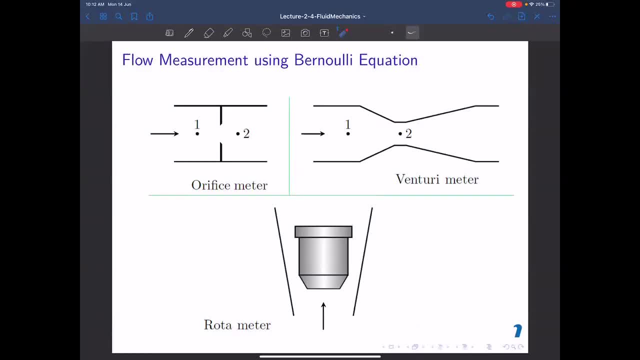 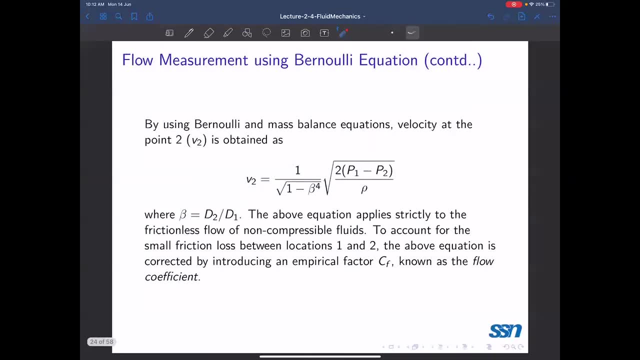 uh, the same thing is also the possible with another device, what is called as rotameter. okay, i will come to this rotameter before. let us see some other idea about this. uh, venturi meter and other thing. so to account for the losses in the between the sections one and two. no, so there is. 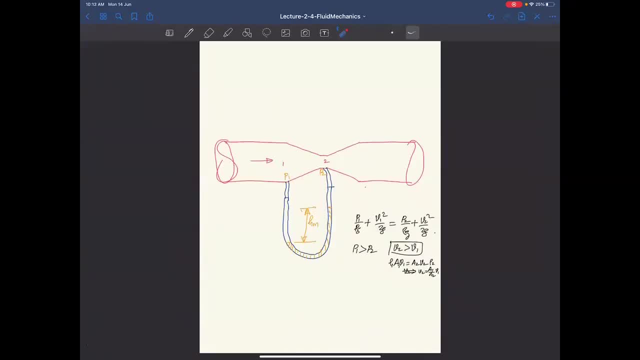 an energy loss, uh, a permanent energy loss, uh, between this one and two. otherwise, because the fluid is reducing in area, i mean the velocity is increased and again velocity is decreased, so the and the friction will be more here. so these are all leading to permanent energy loss. so this permanent energy loss is 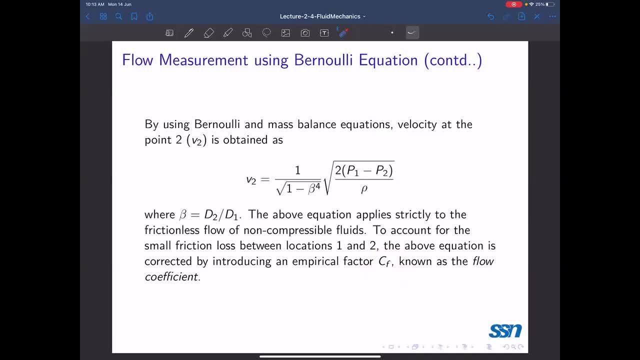 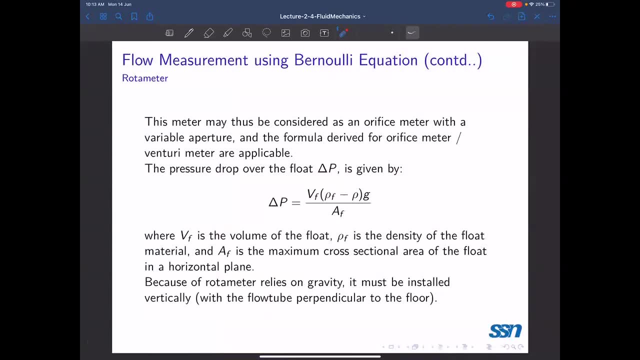 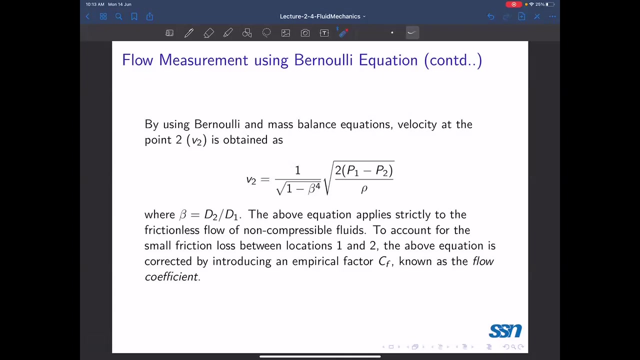 accounted by the factor what is called uh flow coefficient. okay, the major aspects and all we will study in your next course. so this uh. the other device, what is called rotameter, is also using the same uh equation. of this bernoulli equation, say here uh, this uh, according to the flow, this pressure difference. 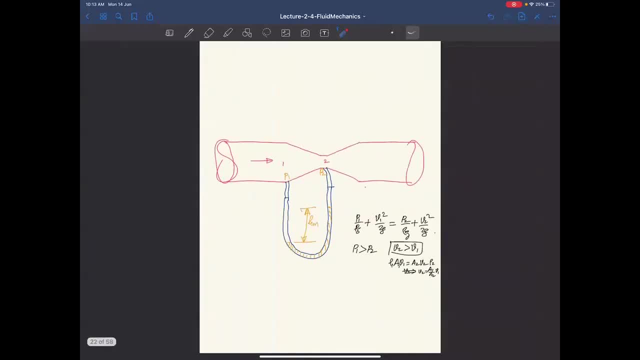 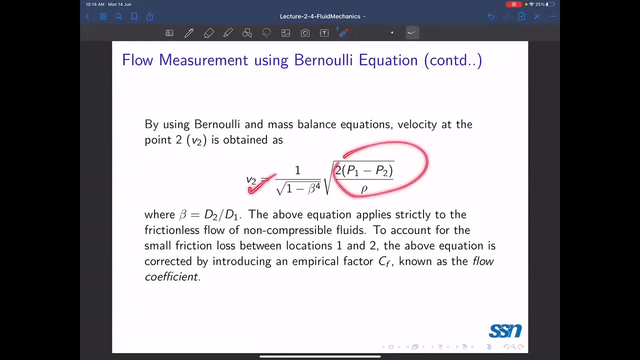 will vary. so, according to the velocity, uh connect to the flow difference. otherwise, if, if there is a higher velocity, higher pressure difference will be created. so otherwise, in proportion to the uh present, in proportion to the velocity, there will be a pressure difference created. so, uh, so the average, the pressure difference is in proportion to the velocity. 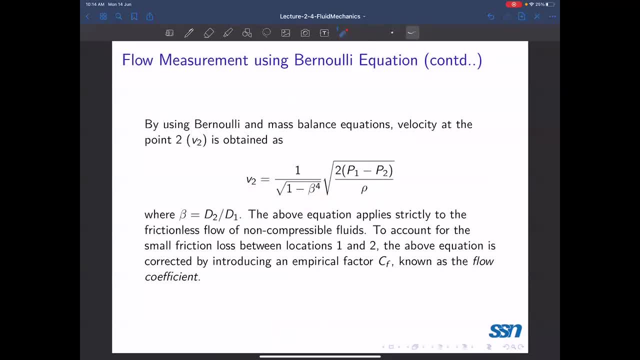 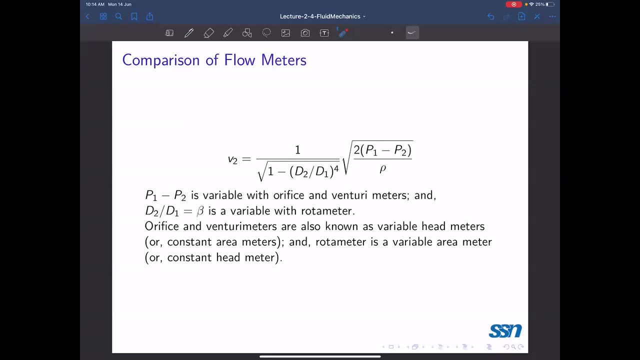 whereas the area of cross-section is not changed. this, uh, this ratio, d2 by d1 for a given construction, this, uh, this thing, is going to remain constant, whereas, uh, the same thing, if you use it for rotameter, the rotameter, this group, this d2 by d1, will change, which is a function of the 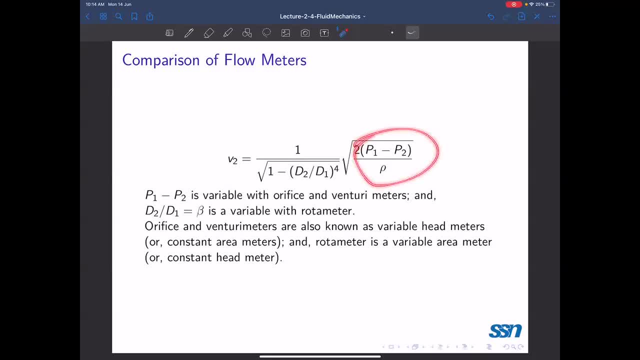 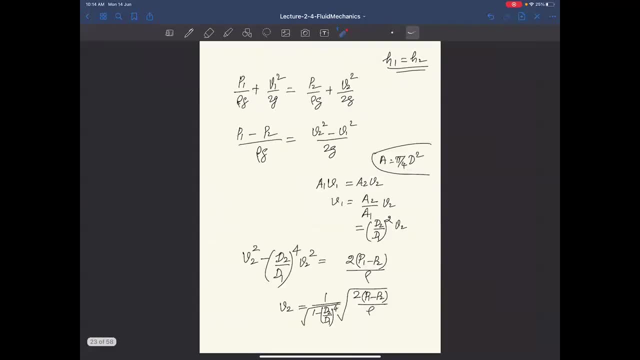 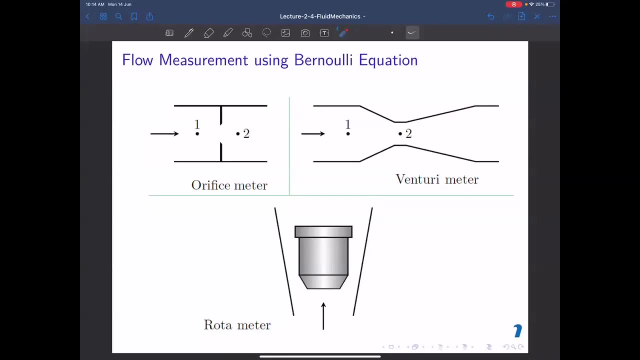 velocity, whereas this p1 minus p2 will remain constant. let us see how that is this p1 minus p2 for the rotameter. let me again coming back, this p1 minus p2 for the rotameter is the p1 minus p2 is uh, or is the p1 minus p2 is nothing but the pressure at this point. 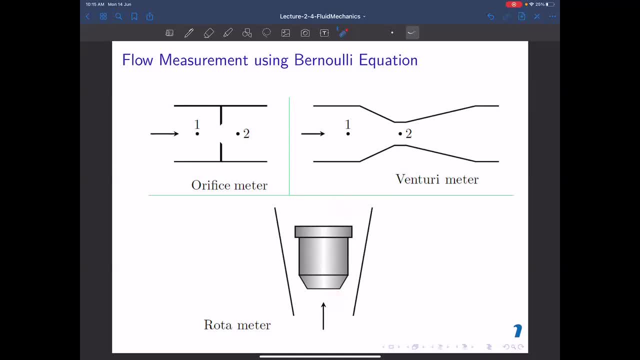 point and pressure at this point, uh, and this pressure difference is, uh, equal to the. there is this pressure difference because of the pressure difference only. actually, this: uh, the float is, uh, this solid is actually floating, actually, the flow, the float is of higher density than the liquid, than the fluid. okay, so if, if you employ water, we'll be having this solid steel ball. 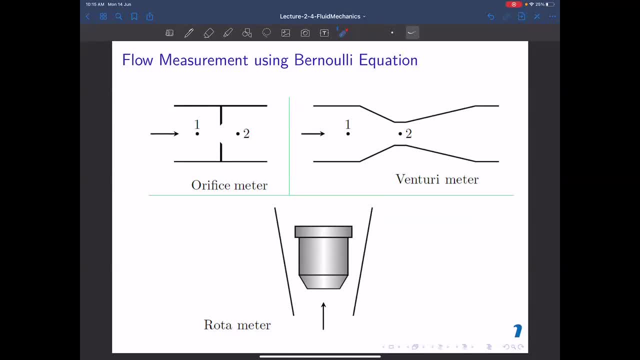 uh, which is floating, uh, this. still, it can't float in the water. water now, uh by, if you see it in the fluid static sense, but it is floating because of the flow. otherwise, it is floating because of the uh, this, uh pressure difference created. there is, uh, this pressure difference is. 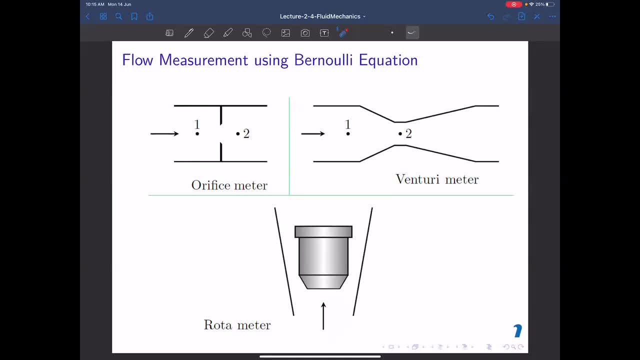 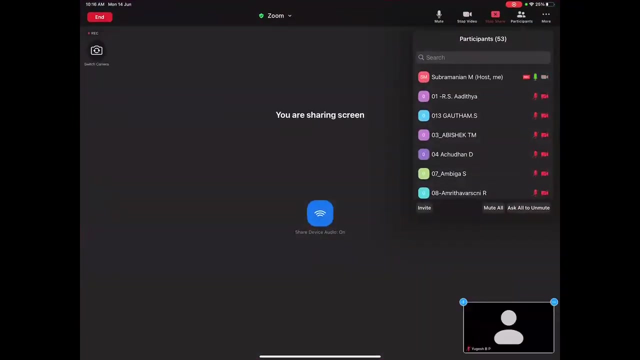 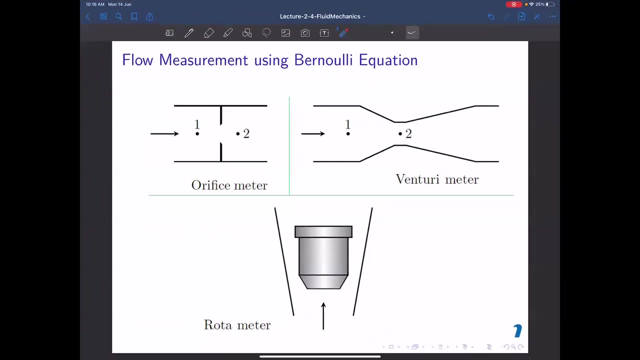 where, because of the uh, there is a inlet pressure because of the flow coming. sorry, wait, wait. so this uh, hope you are following. i'm okay. about 52 people are available, good numbers. so what we are seeing is: uh, we are going, we are applying this kernel equation for rotameter. 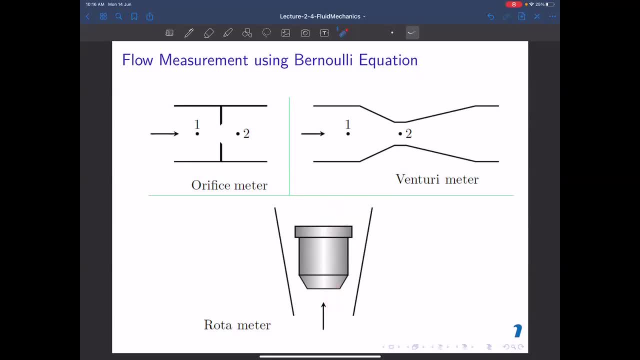 uh, so this pressure difference, of course, uh, in the uh, the float is in suspending position because of the pressure difference. so this, uh, so this is the upward force is uh, uh, there is the. there is upward force because of the pressure one and downwards for because of the pressure two. so p1. 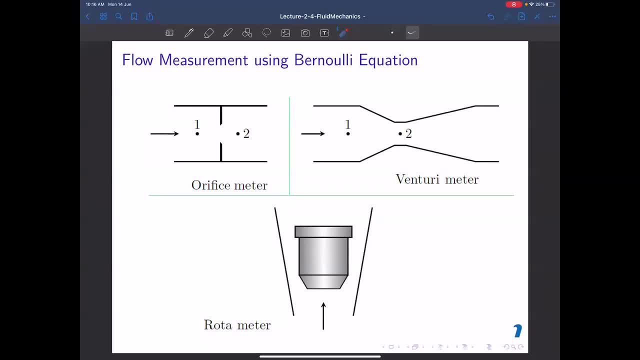 minus p2 is the pressure difference across the float. so there is a downwards meeting supports now natural downwards force because of the gravity of this flow, which is given by mg. m is the mass of the float and g is the acceleration due to gravity, and uh whenever there is a solid in the fluid. uh. 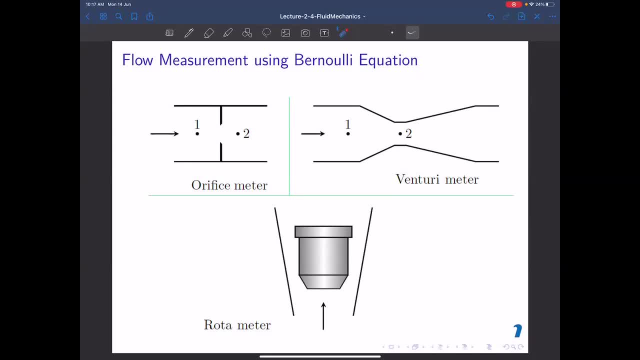 there is what is called a? uh, buoyant force. so even if you take a swimming, swimming in this water, uh, there is a force in that row which we are actually using toこの uh, um, having that force in force opposing your downward flow, what is called as a buoyant force. so buoyant force is equal to. 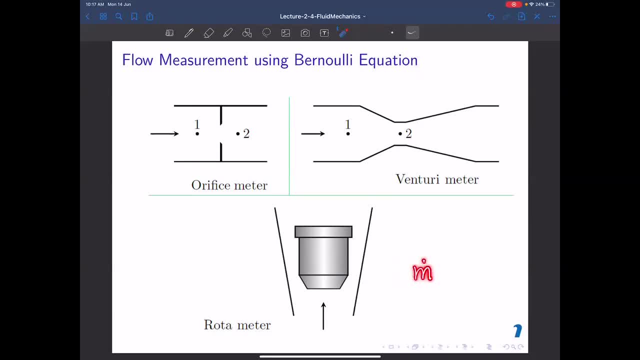 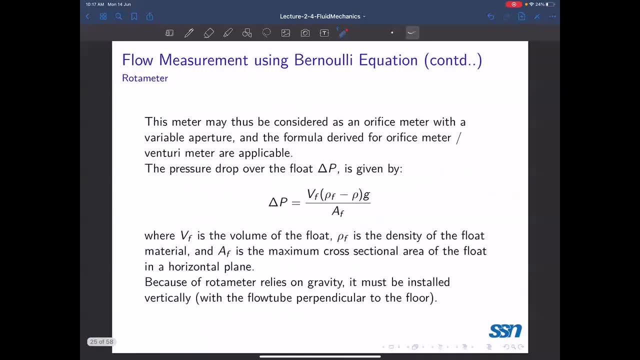 mass of fluid displaced multiplied by density of the fluid. so uh, that thing, we are going to use it now. so otherwise, so uh, this v into rho g, uh v f into rho f. these are all volume of float and density of the float, otherwise m of g. so what is this? 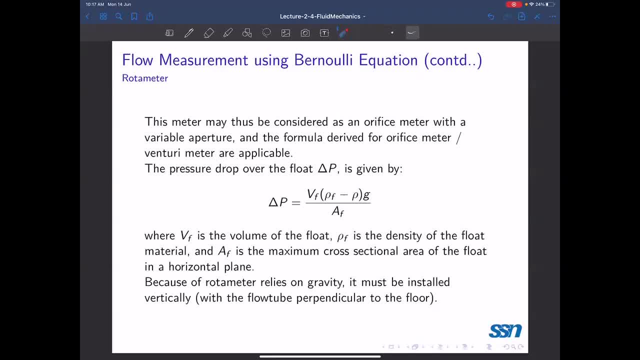 v and rho. v and rho will give you mass. correct v is volume and rho is density. volume into density will give you mass: mass of the float minus mass of the fluid displaced. how do you say this is mass of the fluid displaced? because v of v of float multiplied by rho of the fluid, uh, which 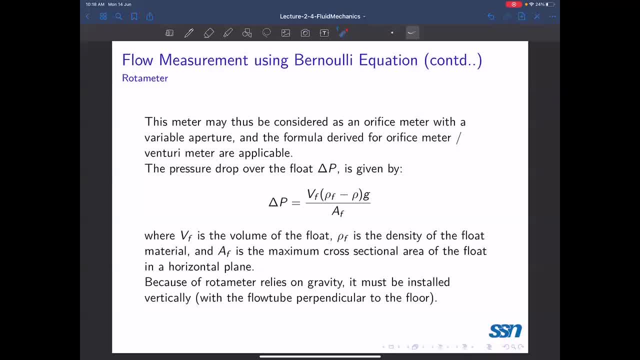 is nothing but the mass of fluid displaced. so otherwise we are getting this. this is gravity, gravity, gravity, the minus is the bands. so there is a net downward force. so this right hand side is the net downward force. uh, delta p is the upward force or is there is a pressure force balance? 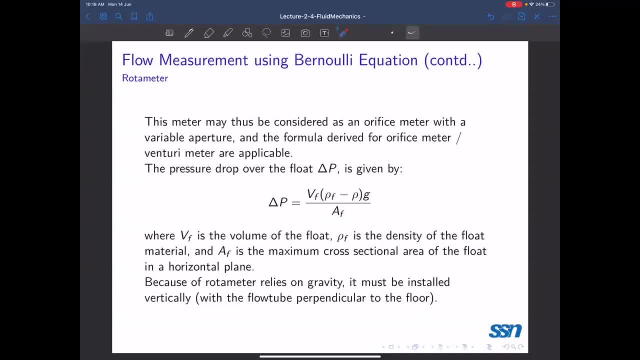 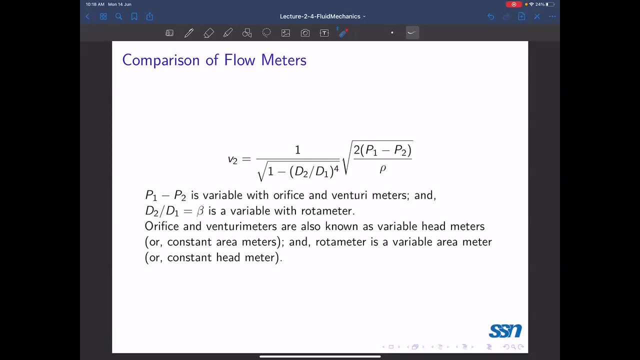 so, uh, again coming back to the. so what is this? a because this is in force terms. force divided by area only will give you pressure. pressure, okay, say uh. coming back to the bernoulli equation: in the bernoulli equation, uh, with venturi meter or orifice meter, there is a variation of this p1. 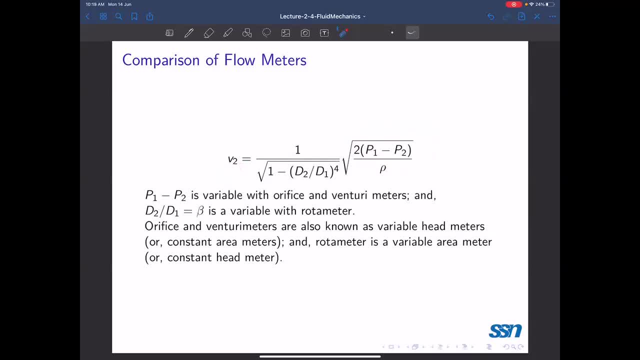 minus b2 in proportion to the velocity. uh, these terms d2 and d1 is a constant for a given cross section of the. for if for a given uh this venturi meter or orifice meter there is, once they are installed, this d1, d2 and d1, they are no longer going to change uh. 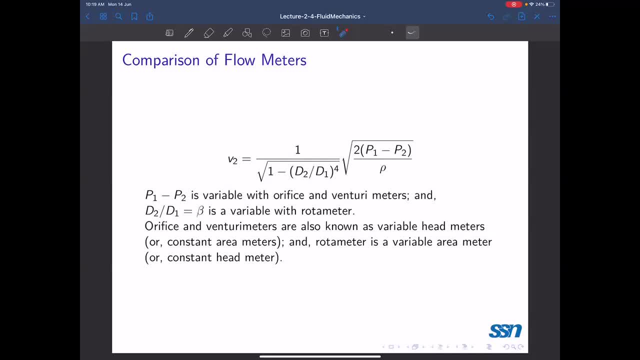 whereas for the rotameter- that is for the rotameter also- we are going to use the same bernoulli equation for the rotameter. this d2 and d1 are going to change, whereas p1 minus p2 by rho- uh, this is a constant, that is p1 minus. p2 is coming from your uh, gravity minus. 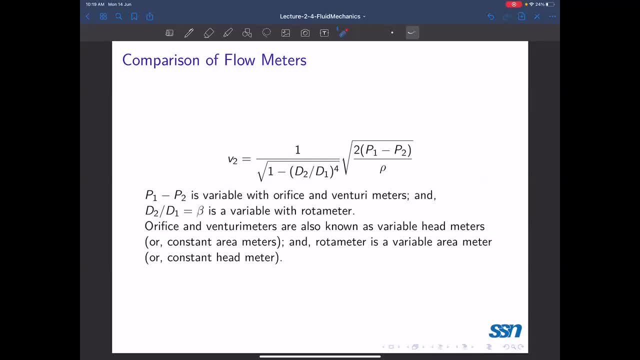 bands. okay, mg minus m, that is gravity minus band force, so that is a constant. of course, the flow of that is caused by the gravity of thewealth band tonight for the manis. uh, there is a method that is called a process or movement of motion across the 2020 thickness of the velocity. Therefore, that motion of mass into the ovenexcम or the different mass of the이었 sitting around spiritim the how, direction violation170010able. but there is an 1988 nap between the carbons and s raft engine over time, the forfeiture and er. so there is a constant sitting and so we call it for relations. 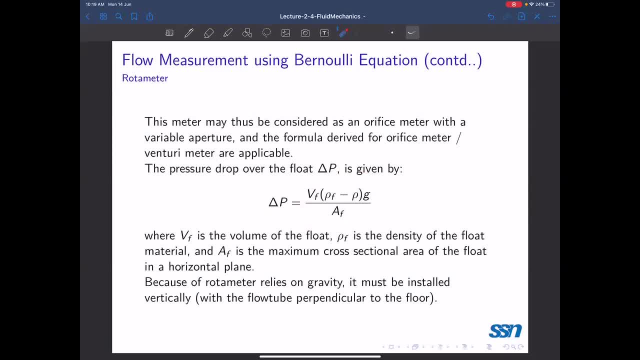 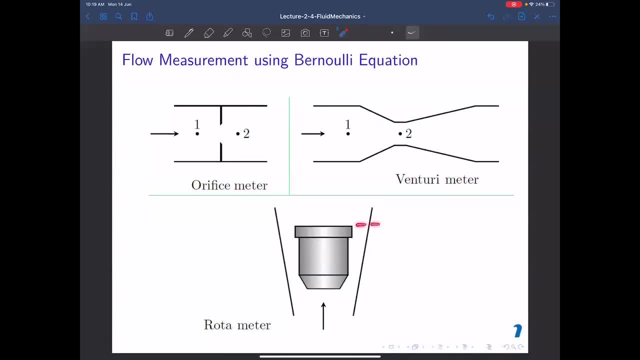 float position depends on the velocity. otherwise, say coming back to the rotameter here, say at low flow rate the rotameter float. if you see that this is a float position, this float position may be somewhere here. otherwise the head no float, the head patina it is at this. 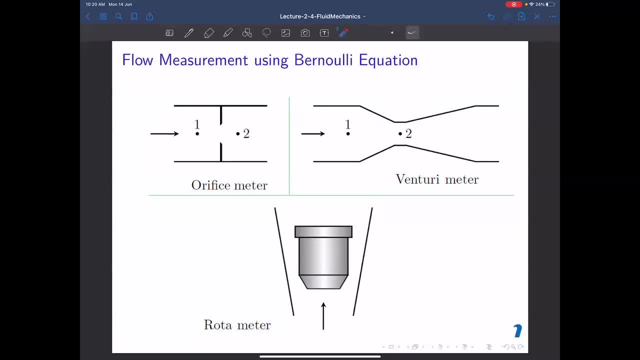 level to start with. it may be somewhere here, so otherwise in that position, in that starting question: what is D2 and D1 here? you can ask now. so D2 refers to the area of this donut now, or is the flow area, or is this flow area available at this portion and this flow area? 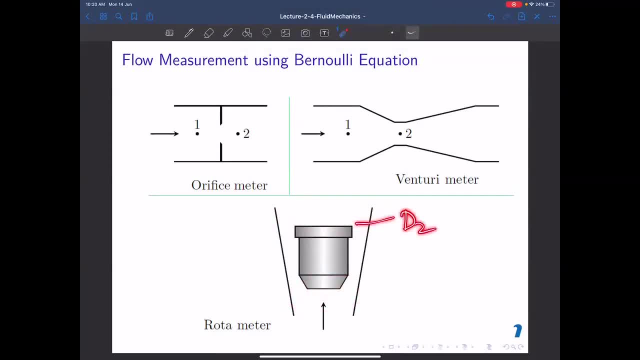 available at this portion. so this D2 refers to this. don't seem say like D2. it is better to say this A2 refers to the area available for flow or that float stop position. Triangular粉术다고this A2 reference to the arolige. you don't see it much in guys. 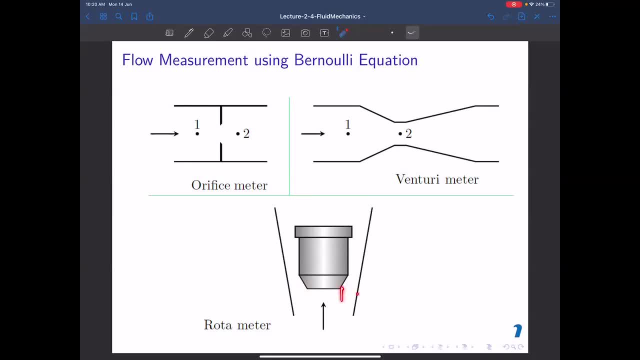 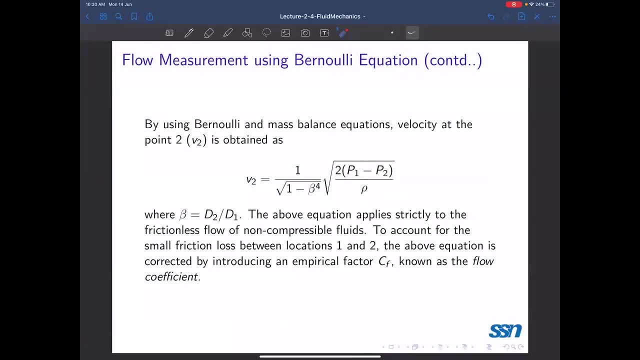 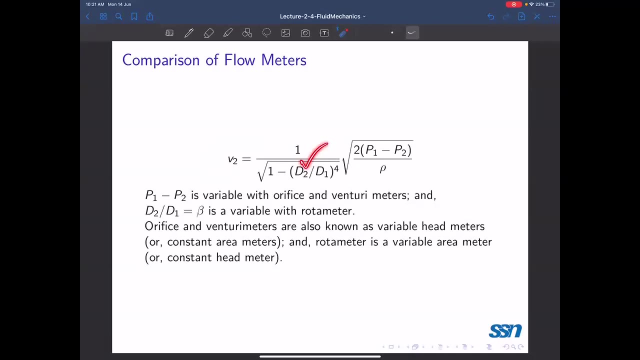 and a1 refers to the area available in the floats bottom portion. so this a1 and a2 are the uh. this ratio is keep on changing according to the velocity. otherwise, uh, according to the velocity of the fluid, this d2 and d1 is varying. otherwise this ratio d2 by d1- is a variable with rotameter. 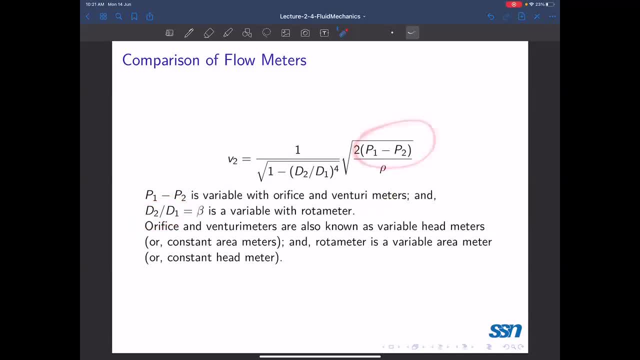 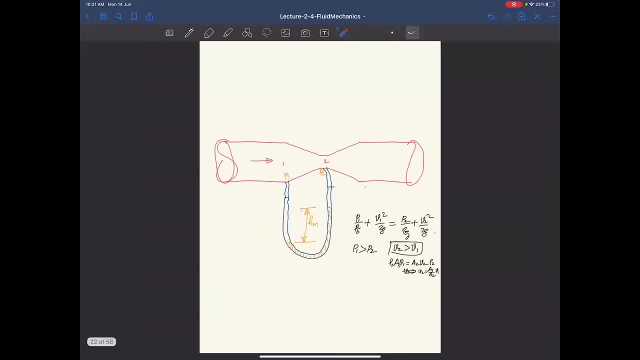 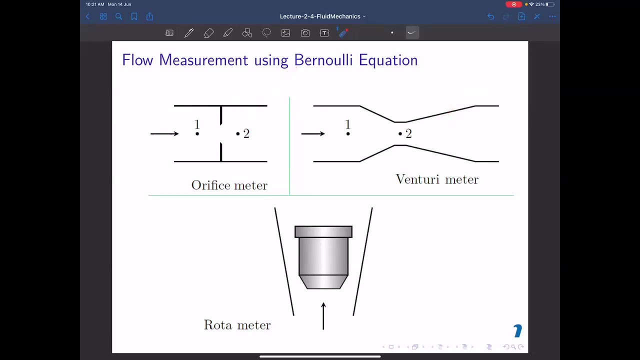 whereas with venturi meter this p1 minus p2 is a variable. okay, are you able to understand this one? the bernoulli equation is applicable for all these flow meters. so this is the venturi meter for which we have derived the equation. the same thing is also applicable for when orifice meter. 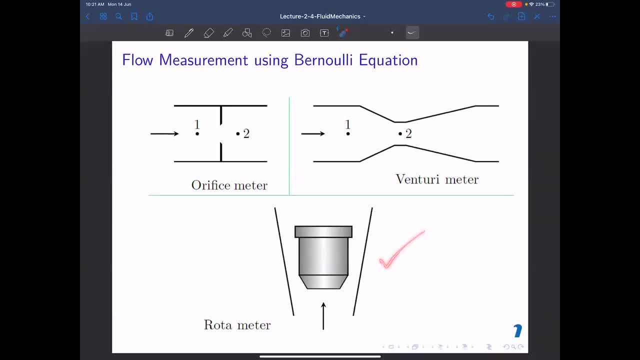 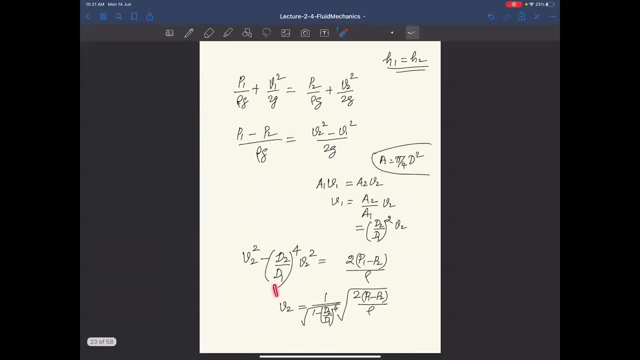 and the same equation you can also imply for rotameter. uh, the difference in this thing is, uh say, out of this equation, uh, the difference in this thing is, say, out of this equation, according to the velocity of the fluid in the flow pipeline, this pressure difference. 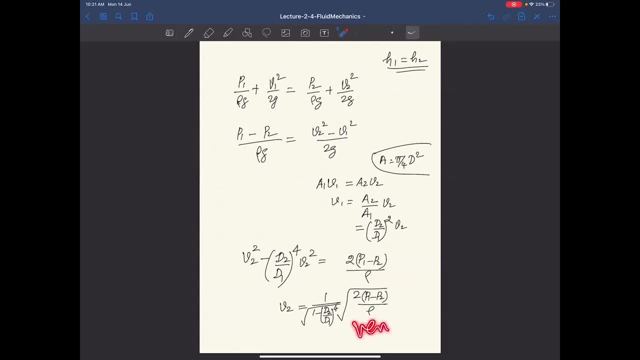 will be a variable in the venturi and orifice meter, whereas with rotameter this p1 minus p2 is a constant uh, irrespective of the velocity, because this p1 minus p2 is simply gravity minus force, so this gravity and biome force is not going to change uh. 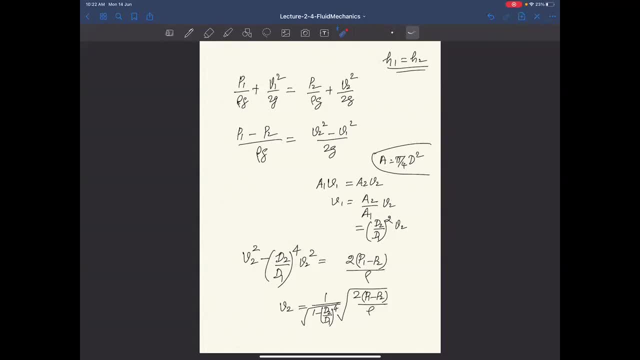 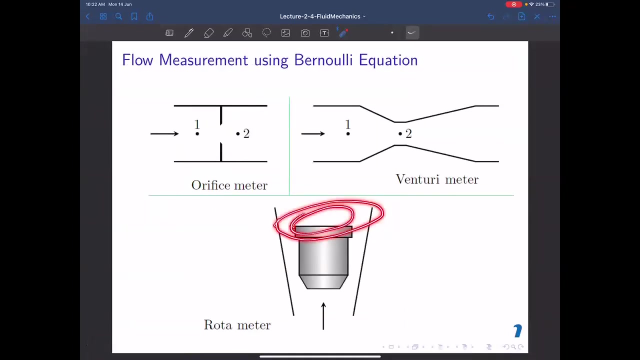 irrespective, it's remaining constant for a for a given fluid. okay, so only this group is going to change. otherwise, d2 refers to the, or we said instead of d2 by d1, you can say this: a2 by a1. a2 refers to the area available for at the top of the floor and here the a1 refers to area, while. 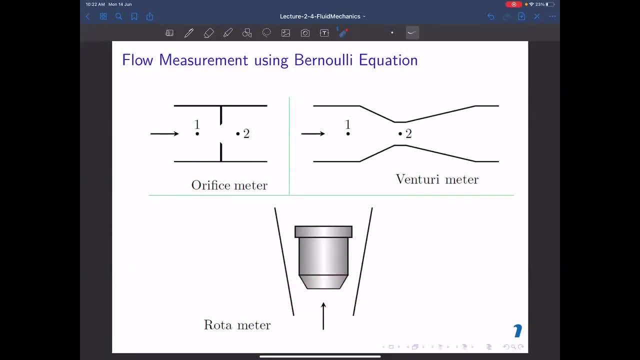 being the bottom portion of the floor. you know this. a2 and a1 are keep on changing. why it change? because of the tap pad cross section of the floor. are this one you are able to change because of the pipeline? okay, otherwise this rotameter, as like this venturi meter, here also we have 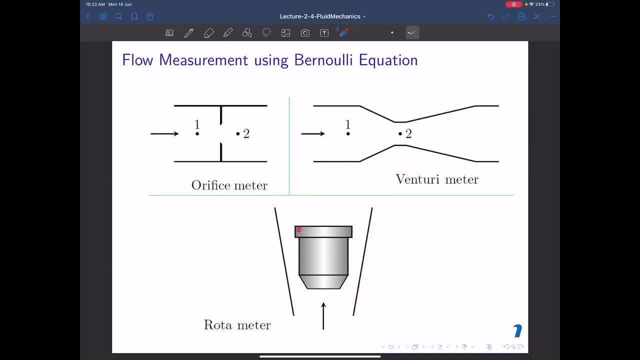 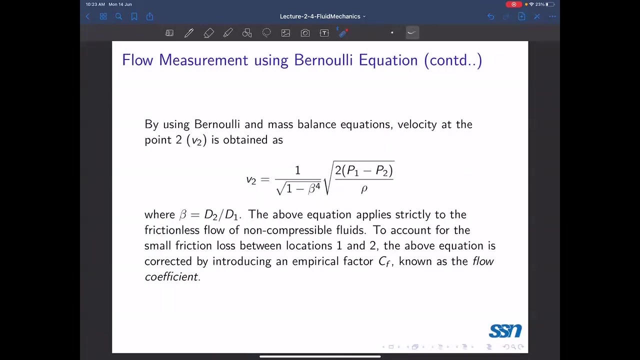 a variable area, otherwise the flow is of constant shape. the flow area is now changing according to the flow, okay. okay, the more detailed aspect you are supposed to study in your fleet mechanics course. at least i can give you a simple idea that same vernal equation is implied for this. 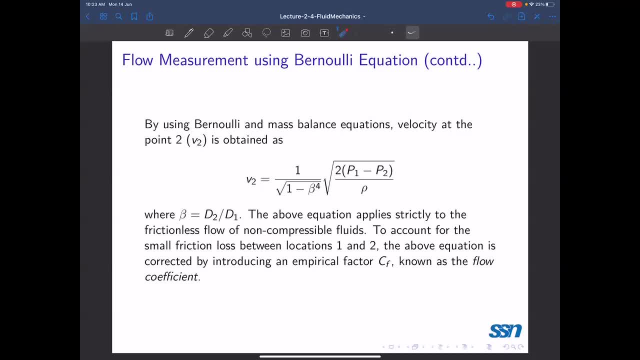 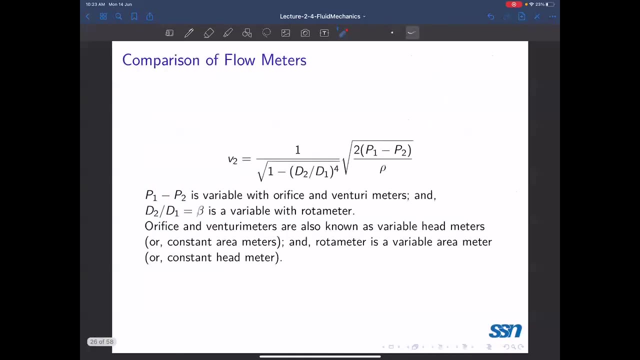 venturi meter or phase meter or what is it? rotameters. so this, the equation, is derivable. you can easily do this. so this is simply coming from vernal equation. okay, otherwise you could see the nice application of vernal equation for flow measurement. it is a summary, okay. 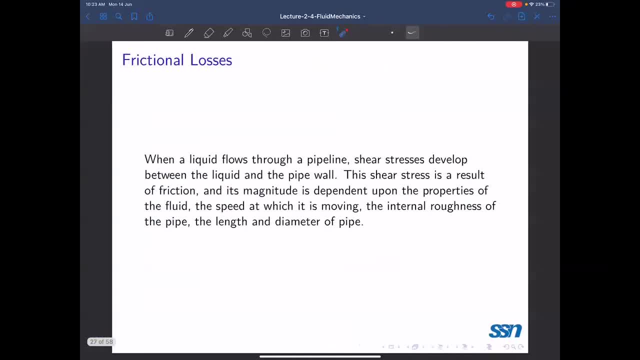 this comparison we have already discussed. now we are going to the next aspect, what is called as frictional losses: how to account for the frictional losses. of course, naturally, there is a friction. whenever fluid is moving in a pipeline, there is fluid. there is a frictional loss because the solid is stationary or the 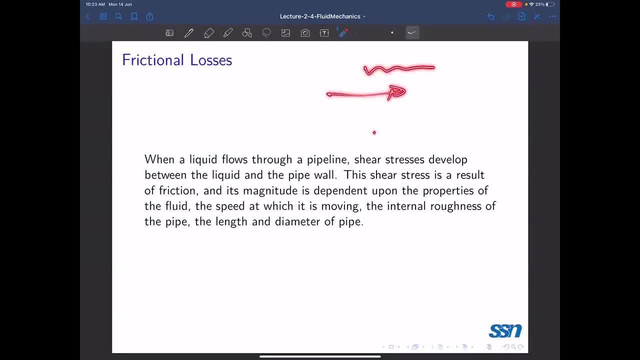 pipeline is stationary, whereas your fluid is moving and there are naturally pipe roughness is there, so there is a loss of energy to overcome the friction between this moving fluid and stationary solid. so what is colors? yes, here. uh, there is a loss of energy by the way of. 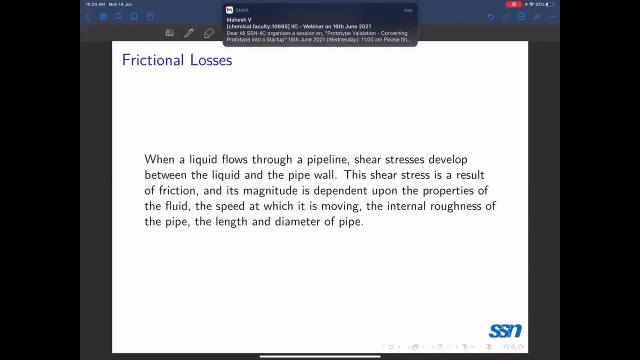 shear force. this is a function of roughness of the pipe and the length and diameter of the pipe. uh, so diameter combination. okay, these things are uh, that is, according to the velocity. there are a lot of factors affecting these uh frictional losses. one is the velocity, another. 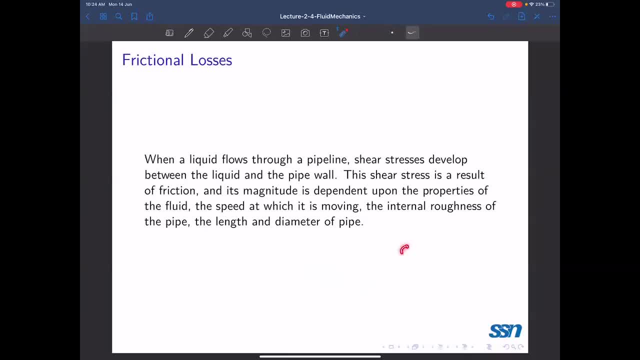 is a diameter. another is the roughness of the pipe, this roughness field term, with this term, uh, e by d. e refers to the absolute roughness, d refers to the diameter of the pipe. otherwise, e by d refers to the diamond roughness ratio. okay, uh, length and diameter. so there are many factors. 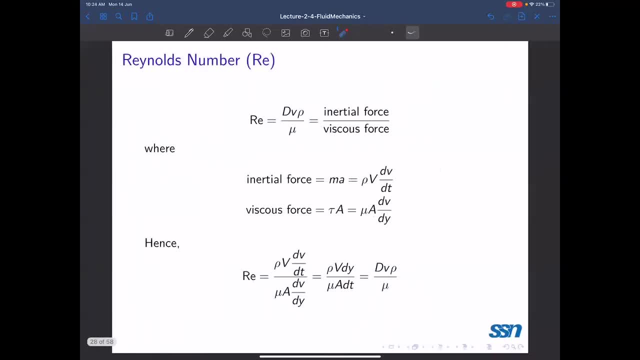 affecting these frictional losses. okay, before coming to these frictional losses, we are going to introduce a new uh variable, what is called as a renal- this very important terminology you will commonly use in your chemical engineering- what is called as renal number, uh, renal's number. it is simply called as a number, though it is a group of variable. 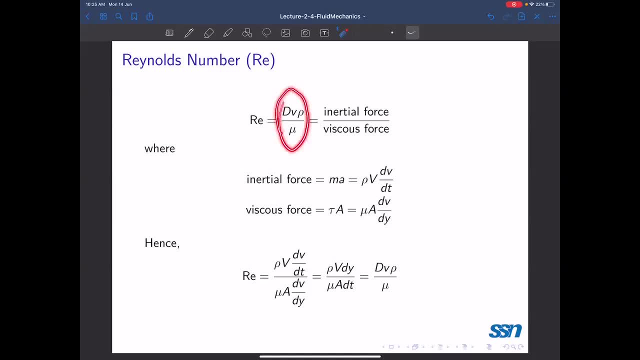 uh, this: variables are arranged in such a way that this group of this variable is leading to a simply a dimensional less variable. that means this group, entire group, will be: we will have no diamonds, or this is simply a number. we can check this also. this dv rho by view. so how this is coming, as dv rho by view, we will see that. 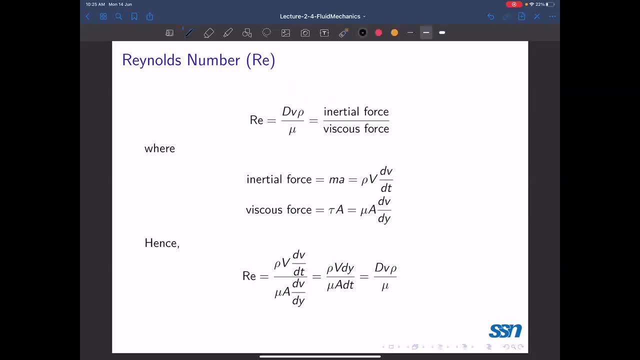 before that, let us check whether it is a dimensionless uh group diamonds or is it should. this entire thing should not have any dimension. uh, what is the dimension of the last diameter? dimension of diametries: meter, meter, fine nice. and v is uh. meter per second. yeah, velocity. 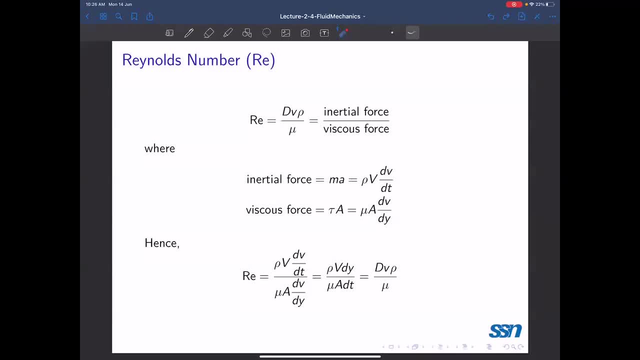 likewise, uh, this dimension of uh density, kg per meter cube, yeah, and viscosity alone- a new thing we have come across. uh, there is in kg uh, or is gram per centimeter second? yeah, there is a fundamental definition of poise, or is ground per centimeter second? uh, it is kg per uh meter second, so you can now check, uh, whether it is. 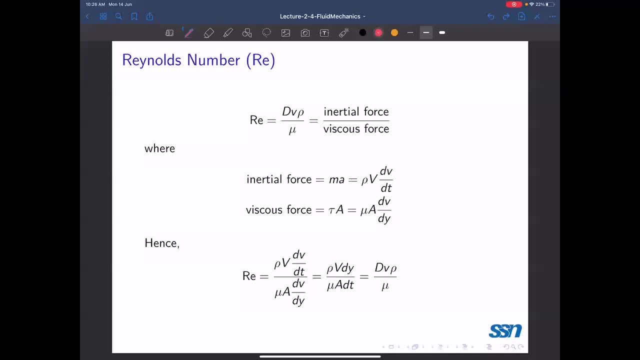 that way you know, uh, let us write it meter. uh, that is for d, for d is in meter. let us take everything in the assignments: and v in meter per second and k? uh, density in kg per meter cube divided by kg per meter second. so now you can see that everything is uh tallying uh, kg, kg and uh already meter square. 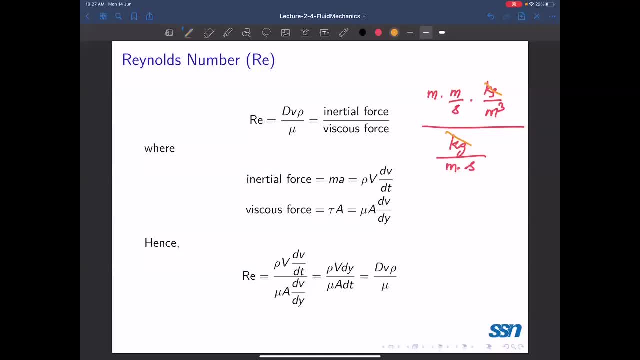 meter square by meter cube. so we'll be having one by meter, so one by meter. so everything is tallying. so otherwise, this uh group, uh, dv rho by mu, uh, we will call it as a reynolds number. uh, this reynolds has worked, uh, worked on this for fluid flow a lot. so uh and uh, this group is called as reynolds number. 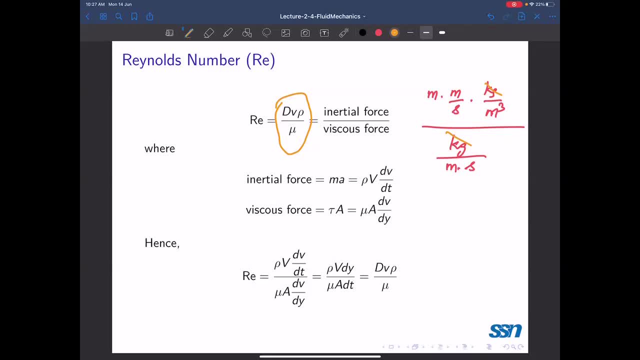 uh, why this group is important and all that. we are going to see it now, otherwise i said about now this uh energy loss due to friction or delta p is energy loss due to friction or the pressure difference due to friction is a function of uh. length of the pipeline, velocity of the fluid flow, diameter of the pipeline. 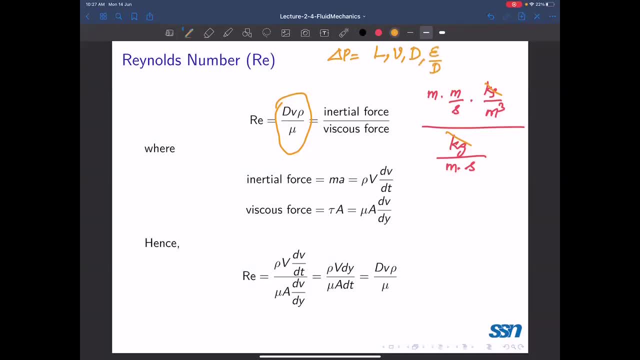 even roughness of the pipe uh in terms of uh relative roughness, e by d was to relative roughness of the pipe uh and what else? even density of the fluid- and of course we can also relate with any other thing also- most commonly they depends on this thing. 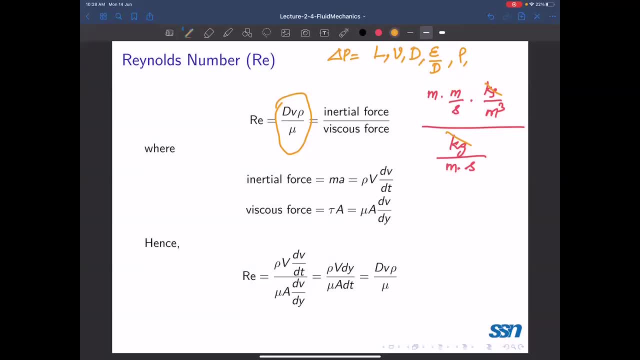 so uh, otherwise, whenever we study this pressure difference, we need to see whether how much is the length, much velocity diameter, whereas lot of variables are affecting this pressure, uh pressure difference, not only pressure difference. most of the uh fluid dynamics variables of importance are depending on this. variables say whether this power required. 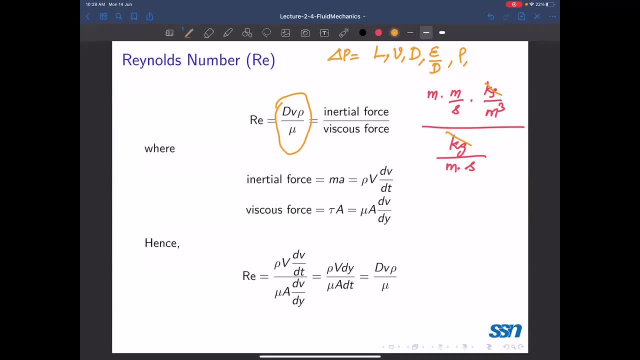 for pumping, or the energy difference because of this friction, all are relatable in terms of these groups. so otherwise, to see the dependence of this delta p, we need to carry out experiments by varying the density, varying the roughness, varying the diameter, varying the velocity and length. otherwise, a number of experiments you have to do, then only you can get the functional. 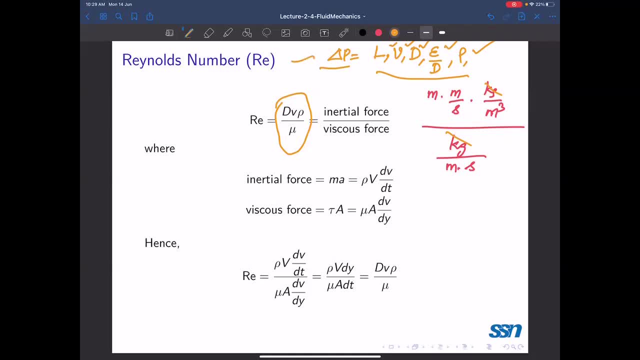 dependence of this left hand side, with the right variables affecting the this group. instead, if you can group these things- that is, we can- if you can group these contents in terms of some minimum number of variables. otherwise, instead of this, d, d, rho and mu, we can group them as a single variable, what is called as a reynolds number. 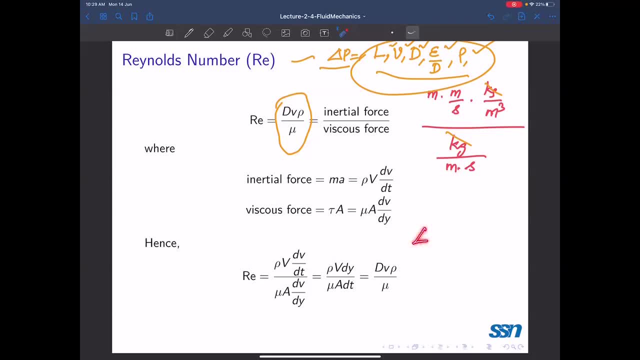 so otherwise, if you want to study the this behavior otherwise, if you want to see the pressure difference because of the flow, you can simply study the pressure difference because of reynolds number. you can simply vary the reynolds number and see how the pressure difference. 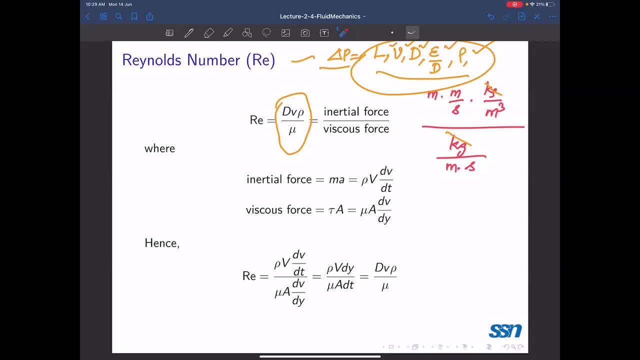 is varying. otherwise, the idea of this grouping this variable is to minimize the pressure difference and to minimize the number of experiments- what is called by dimensional analysis. maybe you have come across this dimensional analysis in your class also. what is called, as you would have related this: uh, you will study in your next course fluid mechanics. that is not complex. 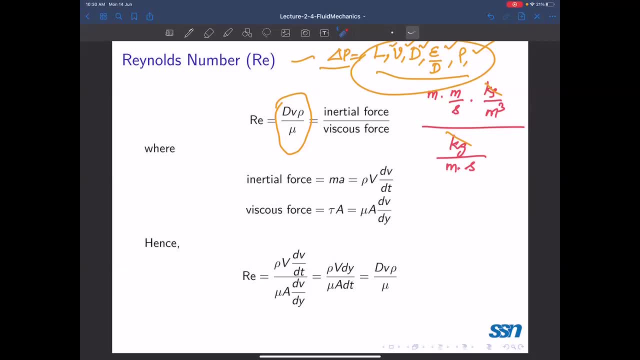 much about that. otherwise, the idea of this- dimensionless numbers- is to minimize the number, is to uh group the variables, uh, in a logical way so that, uh, you will come out with a dimensionless group. so since there is no dimension, you do not worry about otherwise if you use the consistent. 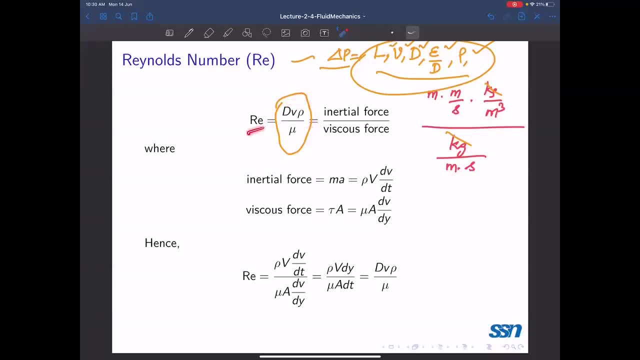 system of units. uh, you do not worry about this reynolds number, so you can simply study the fluid mechanics variable of importance as a function of reynolds number. maybe another, any other group also? okay, so now we are going to see how this reynolds number is going to. 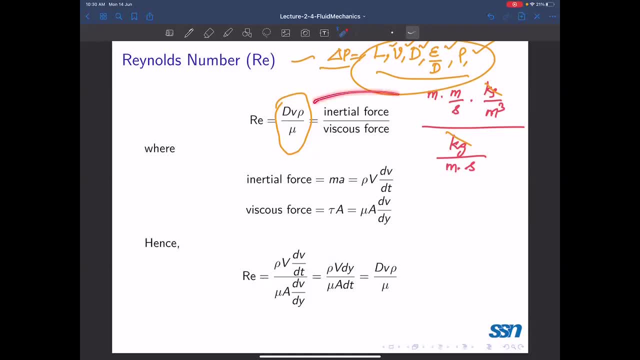 be okay. now let us see about this reynolds number in detail. so this is expressed as a ratio of two forces. let us see how this is coming so. uh, of course, it is set as a ratio of inertial and viscous force. what is the inertial force? inertial force is uh mass into 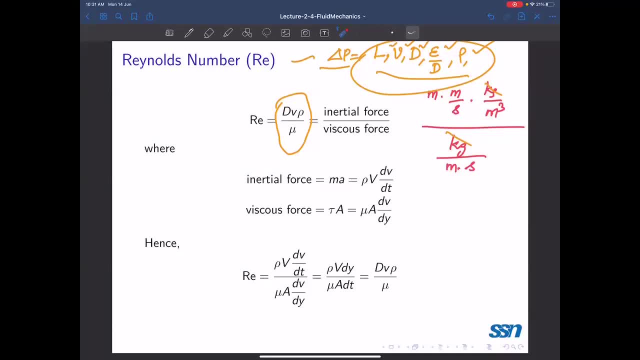 acceleration, uh mass. it can be written in terms of rho into volume, and acceleration is change of velocity. so this rho v into dv by dd is nothing but the acceleration of the nothing but your inertial force and viscous force is coming because of the shear stress. 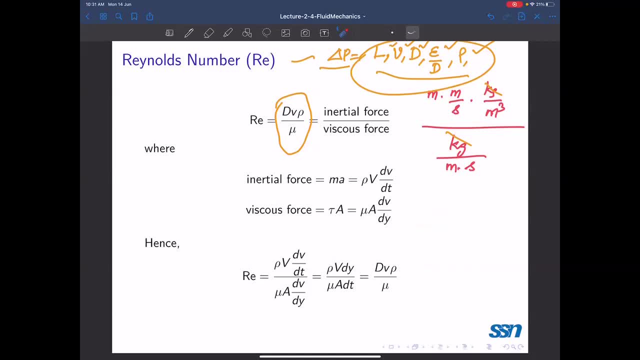 viscous force is because of the viscosity of the fluid. so viscosity- already we know this- tau is proportional to mu into dv by dy. from the newton's law of viscosity we know the relation between tau and viscosity. so otherwise this tau is written as mu into dv. 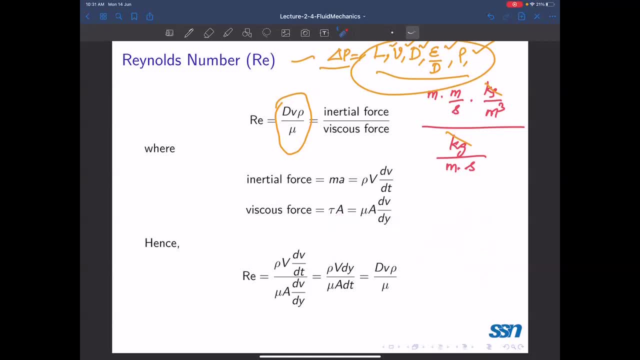 by dy and area is near there, because this is tau, is shear stress and we want to write in terms of force. so shear force is shear stress multiplied by area. so shear force is coming as this velocity gradient, viscosity and velocity gradient. dv by dy is velocity gradient, this is velocity gradient. 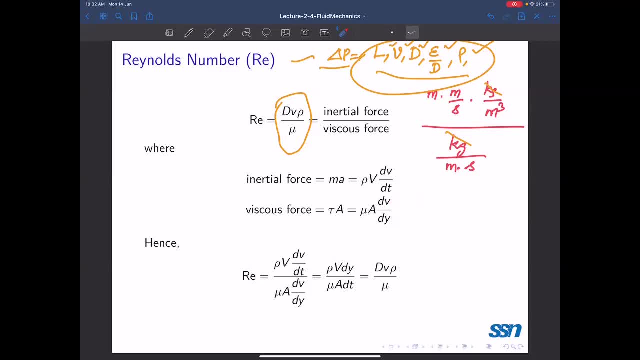 velocity and this is distance. so velocity change the distance. so this ratio, if you take it here, so this rho into v, into dv by d, okay dy, so this dt is still there. so y by t again can be written in terms of velocity, because what is velocity? velocity is distance by time. 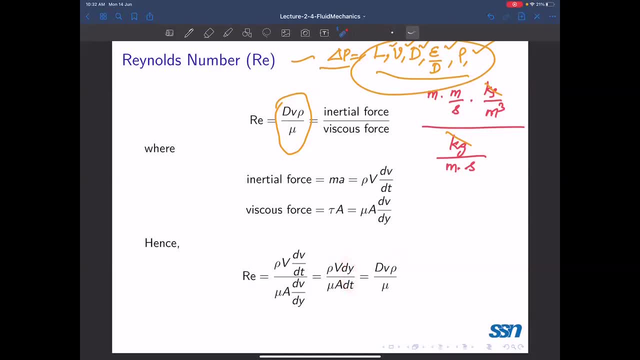 so this is group as velocity And v by. yeah, viscosity is already there and yeah, rho, we need to have v by this capital. v by a is diameter or is one dimensionally correct? don't simply check for this: v equal to 4 by 3 pi r and area 4 pi r square, you won't get this diameter or is dimensionally. 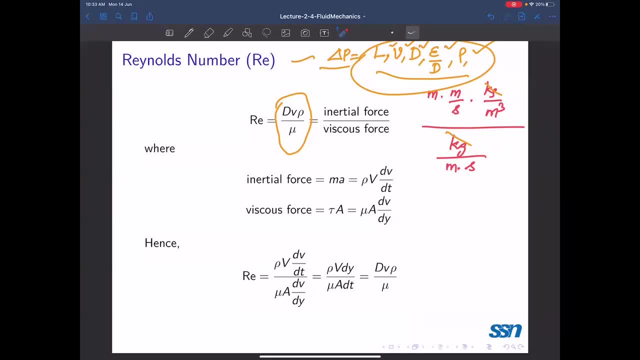 correct. Okay, So volume by diametries, volume by area, is having the dimension of length and u by. sorry, this distance by time is velocity and this is there. so otherwise, this Reynolds number is simply the ratio of two forces. of course, this logically a group of variables, this instead. 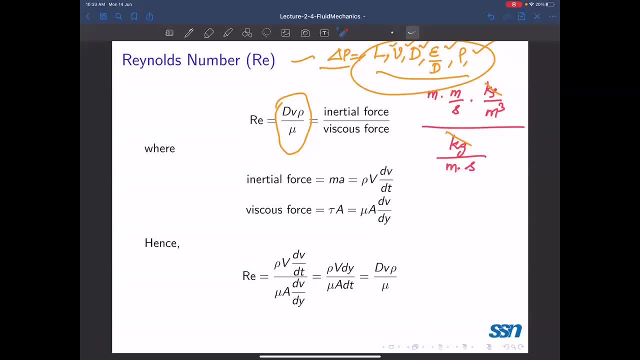 of saying this as variables. you can simply say this in terms of ratio of two forces: one is inertial force and another is visceral force. Okay, If we consider that way, we will again group this flow in terms of two categories: what is called as laminar flow and turbulent flow. okay, we are going to that. we are going to. 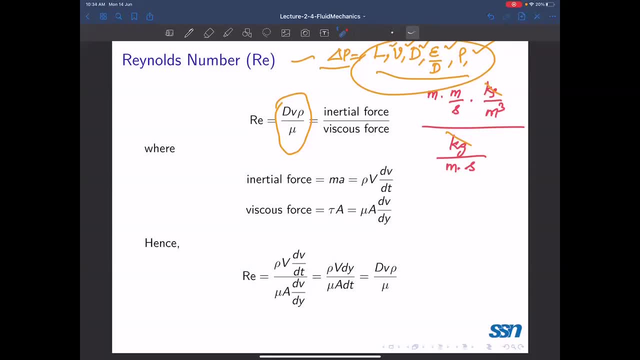 do that shortly. so at least now let us again. check. okay, to again. to summarize this slide, this Reynolds number is a dimensionless group, dimensionless number. dimensionless, that means there is no dimension. Okay, and it is. it is relating the flow variables of importance. so what are the variables of? 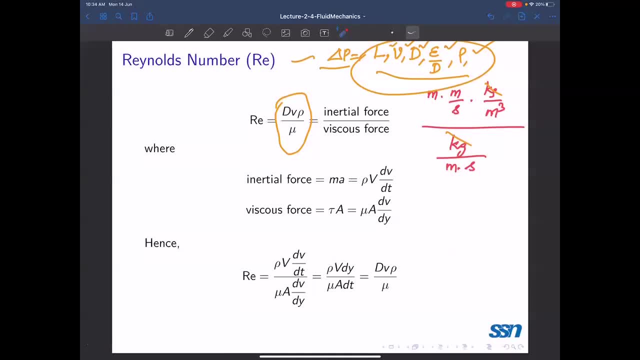 importance. naturally, the velocity is one of the variable predom natural variable of flow is velocity, and viscosity is also another variable affecting the flow flow and, naturally, density and diameter, well as okay, these things are there, which is governing the fluid flow. Okay, now, as I said, we are going to classify this flow. it's a fluid flow in terms of two. 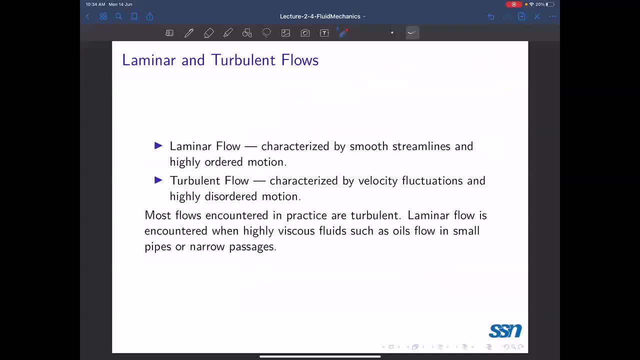 categories. one is what is called as laminar flow and another is called as turbulent flow. otherwise, already we said now this: Reynolds number d, V rho by mu. this is inertial by viscous force, and for laminar flow that viscous force term will be more, whereas for turbulent flow 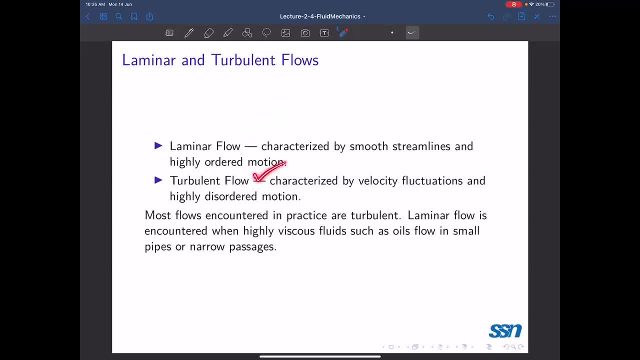 this actually will be the flow, And for laminar flow, the viscous force term will be more, whereas for turbulent flow, this is the flow. Okay, Okay, Okay, this, uh, inertial term will be dominated. uh, okay, uh. how do we say okay? this has to be elaborated. 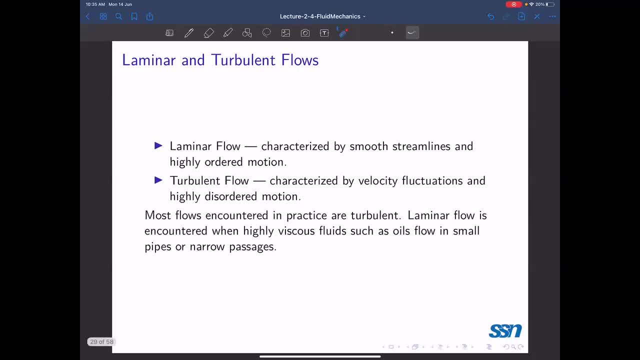 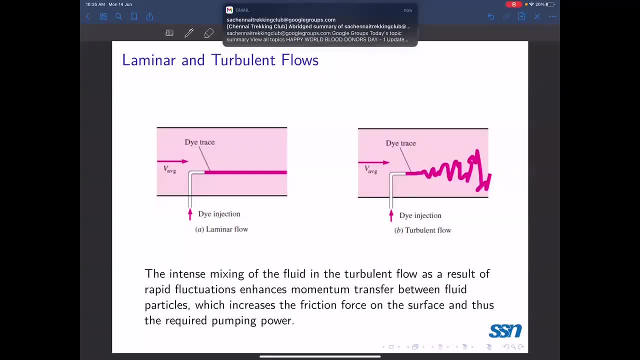 maybe i i can give a simple idea only. so, before that, let us see how this, uh, how how do you identify whether this fluid is laminar and how do you identify this turbulent? see, uh, so assume we have a transparent tube, a glass tube, through which there is a fluid flowing. and if you inject a fluid, 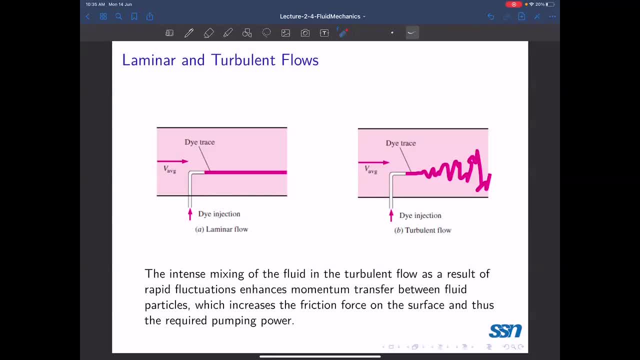 uh, at a point. uh, you can have a colour coloured fluid. so if the fluid is flowing without mixing with the other layers, so otherwise fluid is flowing in this way- uh, you are introducing to it at this point, at a point, the fluid is simply flowing as a straight line. 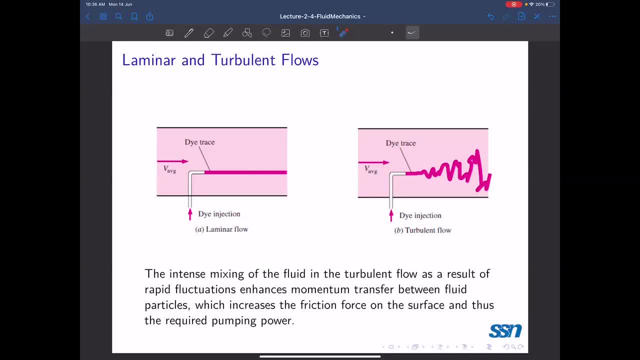 so otherwise the fruits are always. which means, uh, one layer of lead is not affecting the other layer fluid. so what is color? the flow is? what is laminar flow? laminar means yeah, what is it? a plate like flow? uh, you know, you know about this laminates. no, in, uh, this wood industry, they say: like laminates. so these are a flow. 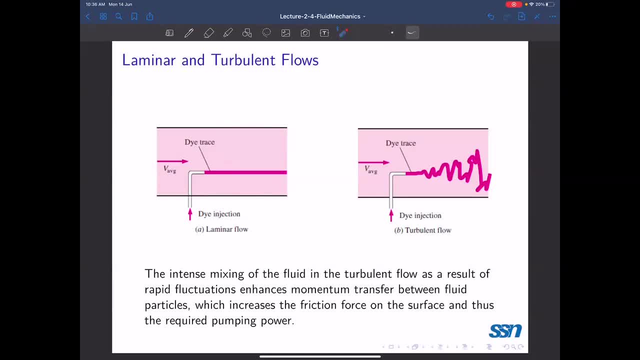 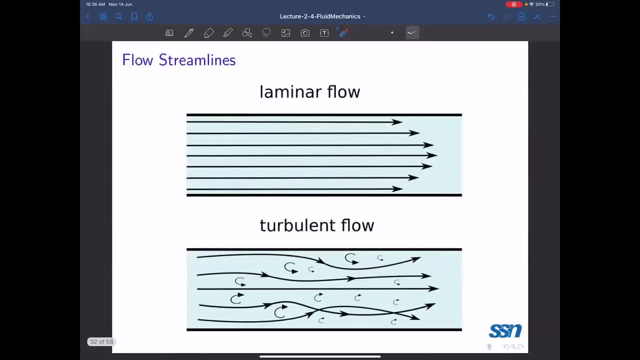 is uh. in a planar flow, one layer of fluid is not mixing with the other layer of fluid, so otherwise free to be uh. i can show you this diagram. so if you see uh, of course the fluid will be flowing in this uh way. of course, you see, there is a difference between the. 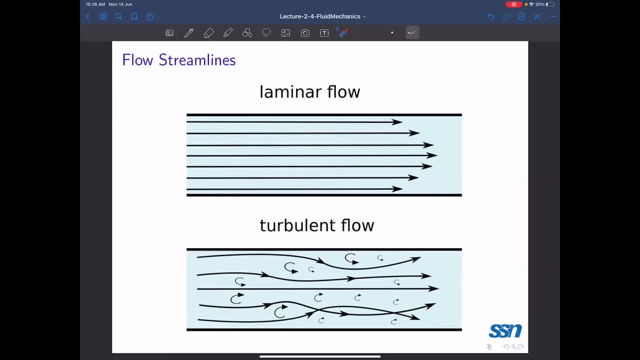 ro head service. uh, this is to indicate that the fluid in the center line will be moving at the maximum velocity. the fluid closer to the pipeline will be almost at zero velocity. uh, that means you can see, you can say, you can nicely make a diagram, what is called as. 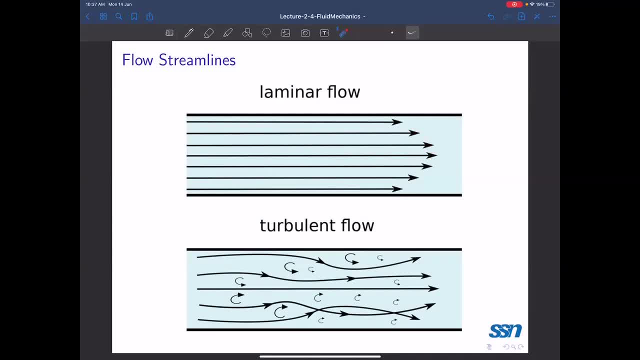 a parabolic profile can be drawn, uh, which is indicating the uh. what is it? the velocity profile or velocity variation with respect to the radius or the distance velocity profile. so velocity profile is found to be a nice profile which is a parabolic profile, will be there with laminar flow. otherwise, if you inject a, if there is a part, fluid particle. 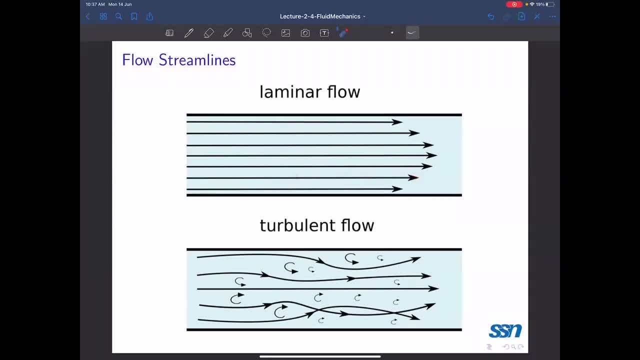 here, it will simply flow in the same line. uh, it won't go to this next uh stream, but these are also called some lines, what is called stream lines. let us not confuse you. so this, uh, this flow is in a happening, orderly, whereas in turbulent flow. uh, whatever the fluid you inject, that point it will simply go to the. 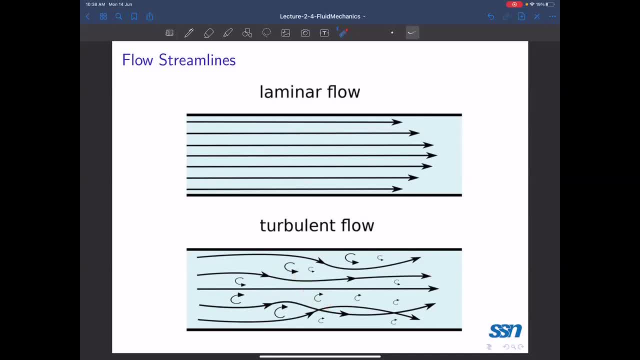 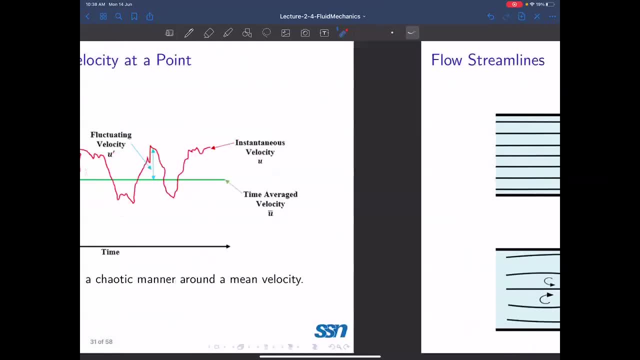 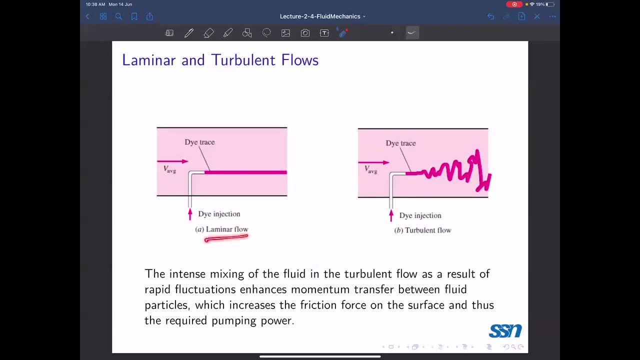 other layer and again come down. so otherwise you will have- uh, i will say it is not a orderly- orderly flow or this will be having a chaotic flow, uh, so this difference is: uh, the flow initially is at low velocity. the flow is normally, in this laminar flow situation, at high velocity. 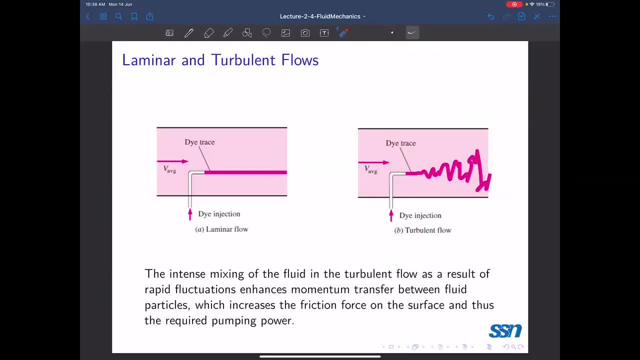 of fluid. you will see the uh. there is a mixing created, what is called the fluid layers are mixing, so this is what is called turbulent flow. you would have seen this, those who are uh smoking and uh, if you see the smokes, uh at, uh to start with, it will come in a nice, orderly wave. 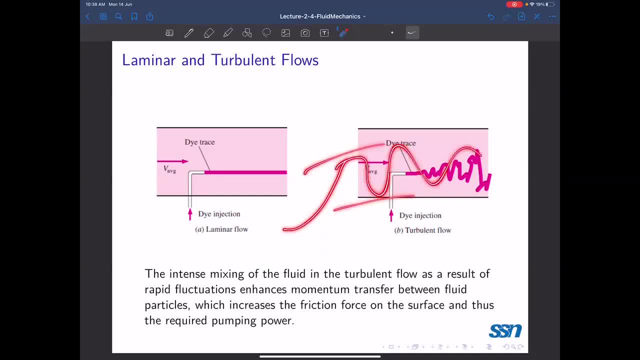 and because of the air surrounding here, it tends to mix up. so otherwise, uh, it will be again mixing. otherwise, at low velocity, you can see this laminar flow to prevail not only in low velocity. uh, there are a lot of other things affecting and, uh, always, these things are grouped in terms of what is. 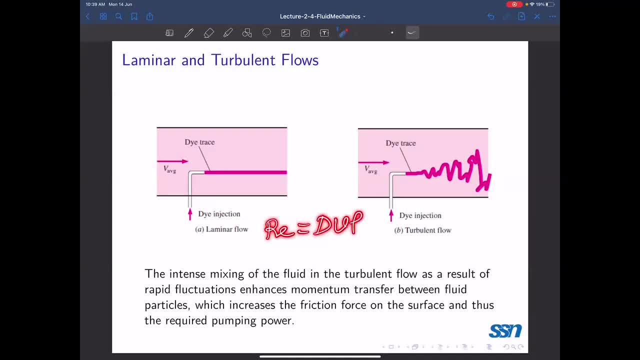 colors number, which is d v rho by mu at low velocity, definitely you can expect low reynolds number. so otherwise, at low reynolds number to be precise, to clearly say the laminar flow will prevail. uh, whenever the reynolds number is lesser than about 2000, or even sometime in the books you have seen, 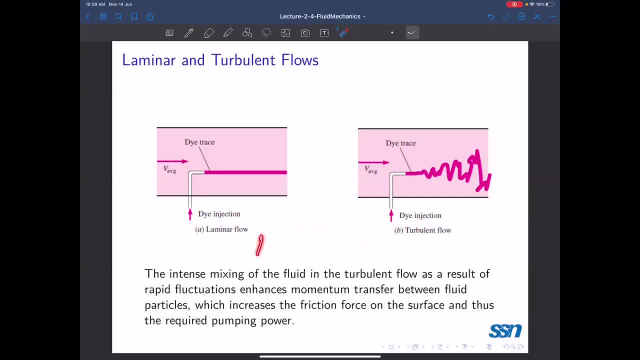 us, you would see us- reynolds number of 2100. for reynolds number lesser than 2100, the flow is going to be laminar- uh for high, uh for flow, uh for reynolds number higher than about four thousand and the flow is naturally turbulent. there is a mixing of fluid layers in between two thousand. 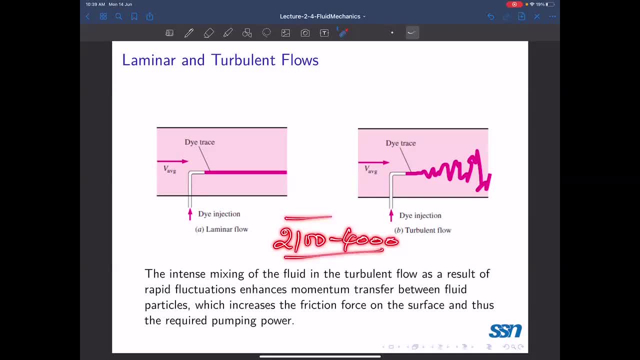 hundred and four thousand, uh, according to the level of disturbance. okay, uh, otherwise the region between two thousand hundred and four thousand is uncertain. uh, sometimes we can maintain these and then the flow will be laminar at that level. so otherwise, below two thousand hundred, this flow is definitely laminar. above four thousand, four thousand flow is definitely. 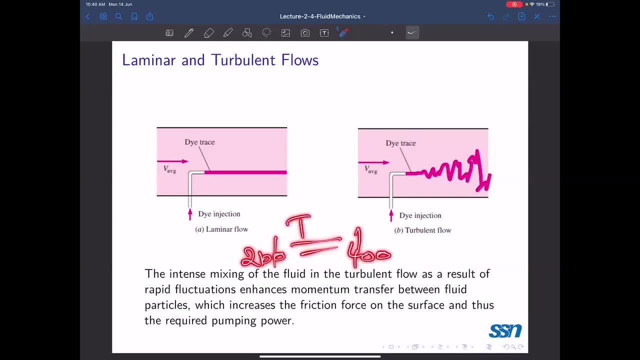 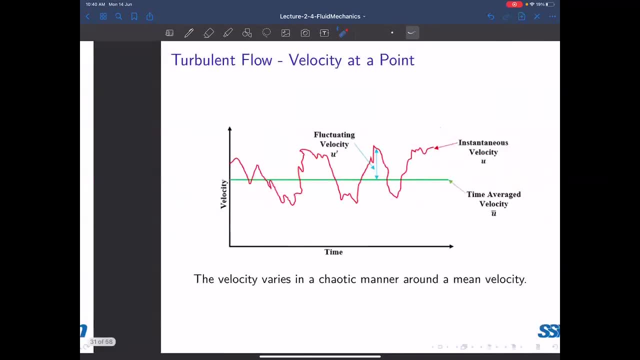 turbulent in between these uh, two thousand hundred and four thousand, uh, what is called a set transition region transition. okay, we have to elaborate in the coming class instead of finishing these. frictional aspects, frictional losses: okay, uh, to summarize today's uh discussion, another about five minutes is enough for the previous lecture, uh, so now we will be back with a. 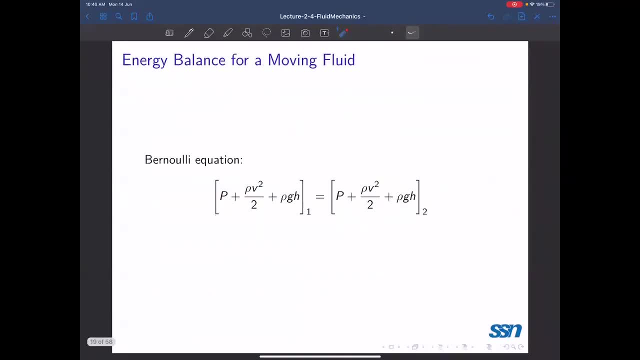 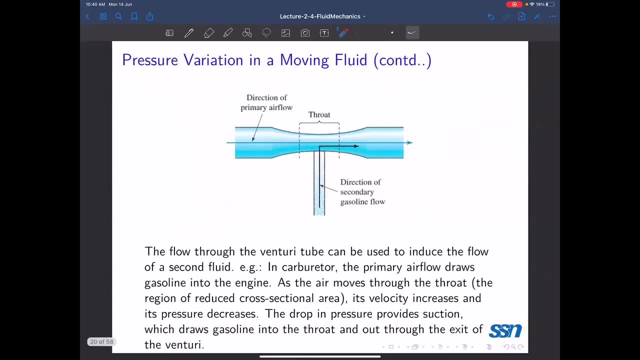 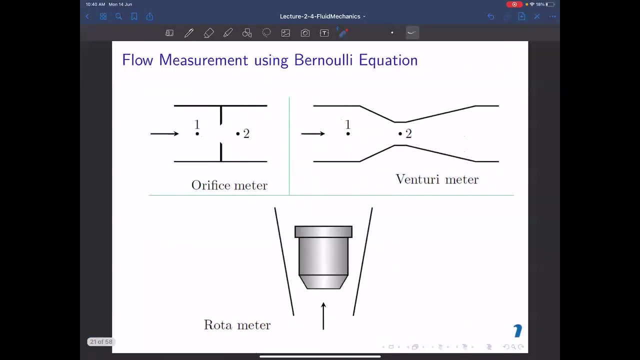 minutes really left. so to summarize today's discussion we have seen about this application of bernoulli equation for flow measurement. the simplest flow measuring devices are venturi meter, orifice meter and rotameter. venturi and orifice are simply by putting a reductional, reduced cross. 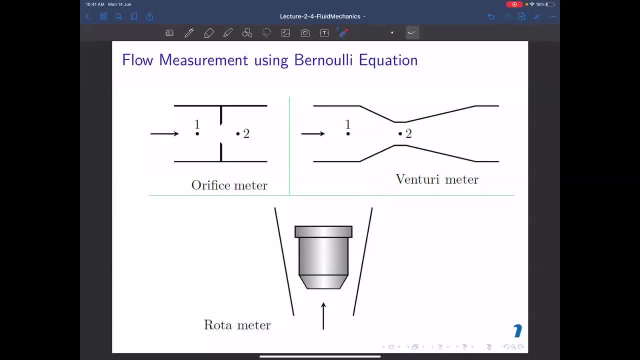 section and measuring the pressure difference across the cross section, whereas in rotameter we have this tapered cross section tube. of course, this tapered cross section normally a glass section so that we can locate this float stop position and this float top portion will be measured with the scale and this, from the scale reading, you can measure, estimate the flow, okay. 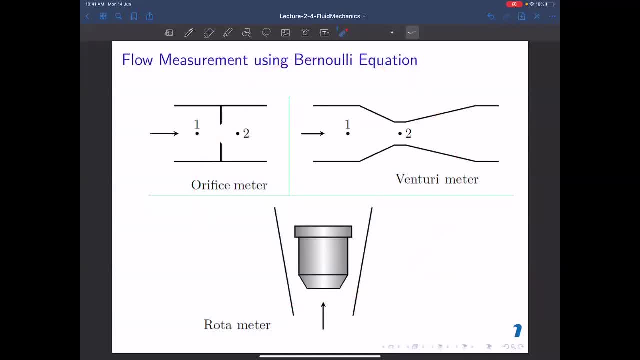 so this, all this device, three devices, not only three devices. there are again variants to these devices. so these are all to measure the uh flow of your fluid flow. is actually this volumetric flow? volumetric flow again can be uh converted in terms of mass flow because you know the density of the fluid, or is 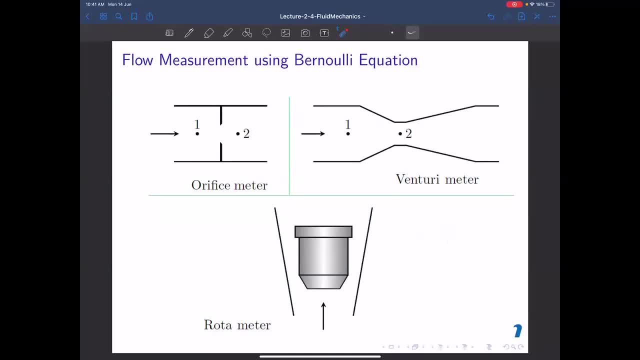 actually we are measuring velocity. velocity is again in terms of volumetric flow rate and yeah, and you can get via mass flow rate as well. okay, and with this orifice, venturi and these two meters are having the same kind of principle: rotameter with rotameter, this flow area is varying, uh, whereas with orifice and venturi meter, 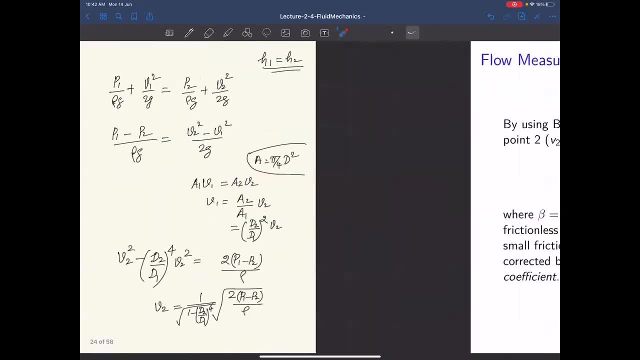 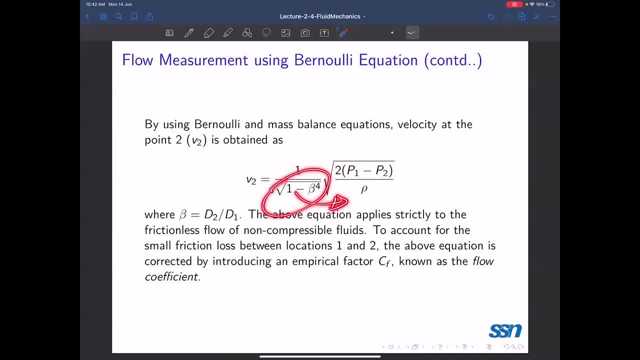 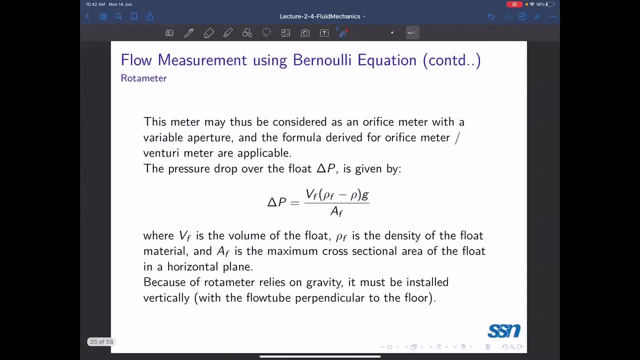 the pressure difference is varying. so otherwise, if you see the equation, uh, this group is varying for venturi and orifice, whereas this group is varying for rotameter, otherwise varying with velocity. okay, okay, this is all we have seen, uh. next, we have uh discussed about this. uh, grouping of variables in. 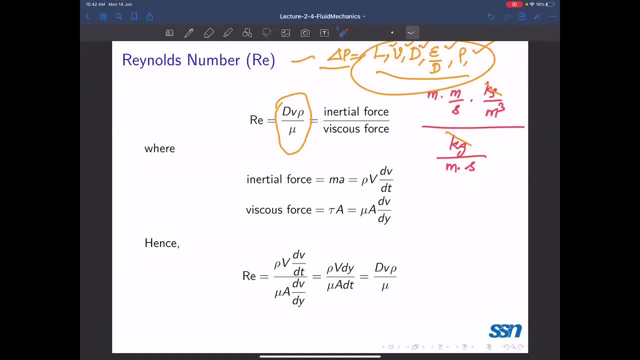 the fluid mechanics, the, the most common uh dimensionless number you would uh naturally use in fleet, not only in fluid mechanics. this you will also use in heat transfer. not only in heat transfer and as well as in mass transfer also. you'll use, so otherwise this reynolds number, which is simply logical. 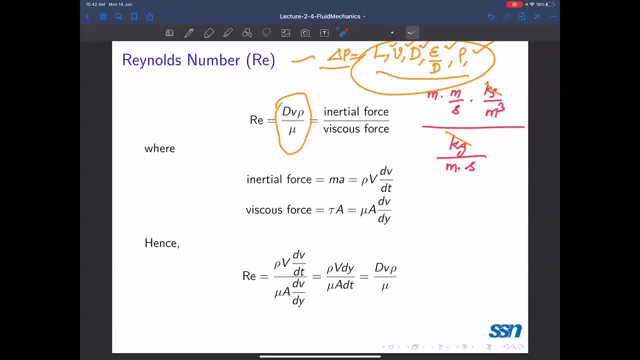 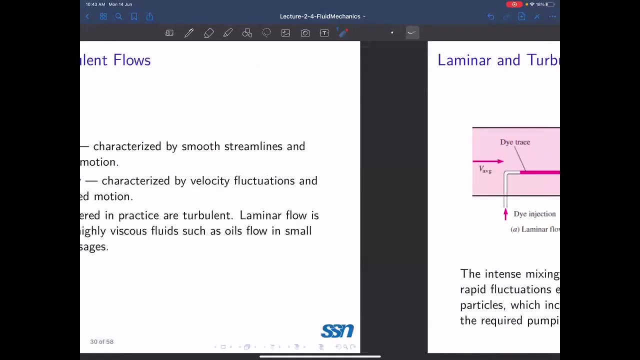 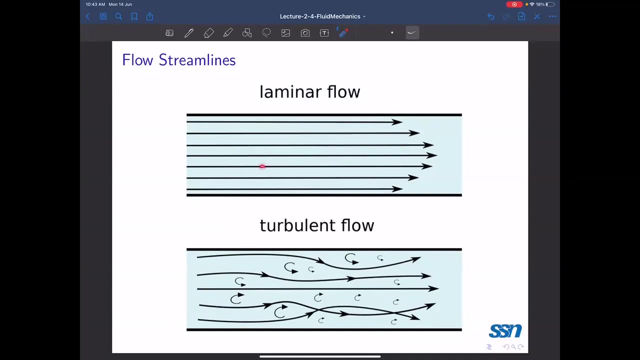 grouping of variables, uh, so that you are getting a dimension less. number this. all these variables are affecting the fluid flow and we have seen about this laminar flow, which is about smooth stream lines. this stream line refers to this line of fluid, these fluid lines, uh, if you have a particle, 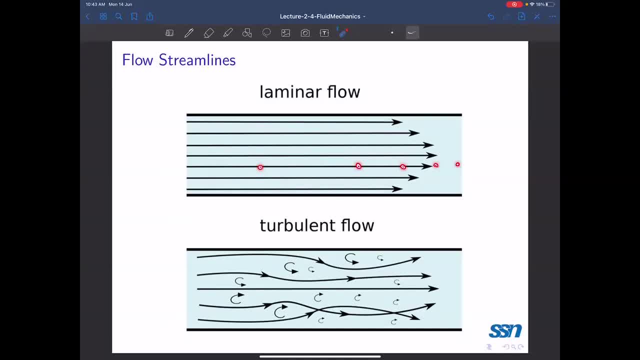 fluid particle, injector particle. here it will move on in the same uh line, provided there is no change in cross section. if you reduce, reduce the cross section again. uh, this flow stream lines may merge and again diverge- convergent diverts- whereas in the turbulent flow we don't see such a nice streamlines. these streamlines are again mixing, or is we see? 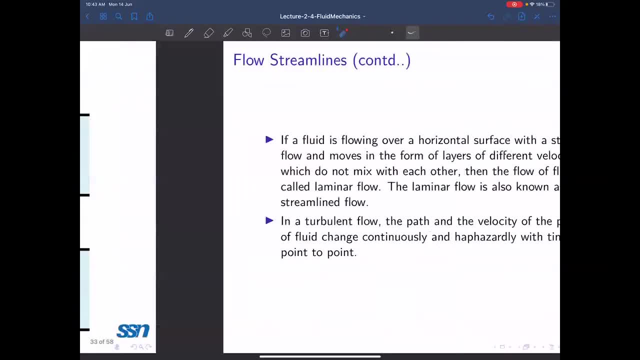 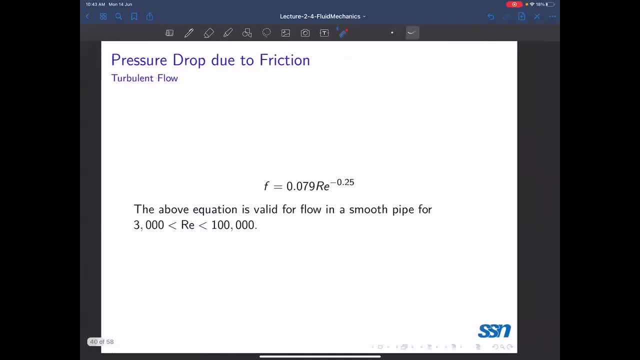 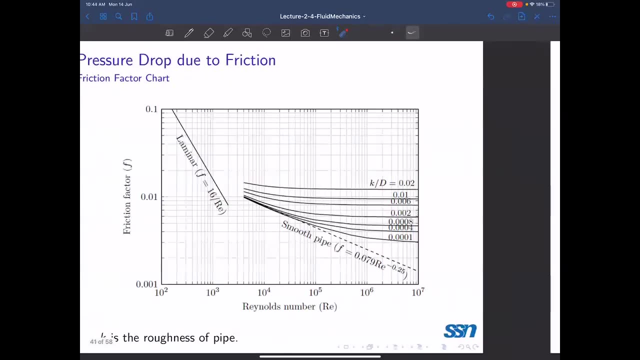 what is called as a chaotic flow. okay, these are all we will elaborate in the coming class and in the next class we will see about the how this friction is accounted in the. this is how to estimate the friction and how to account for. this is how to over, how to supply. 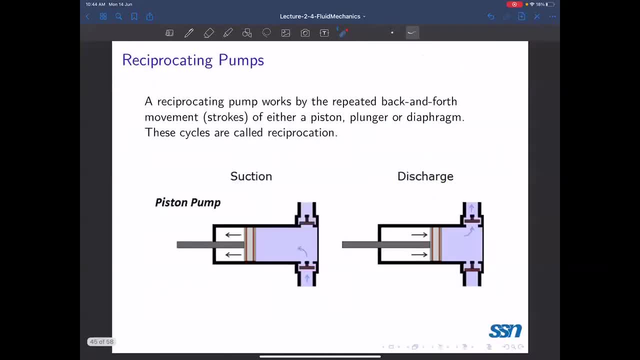 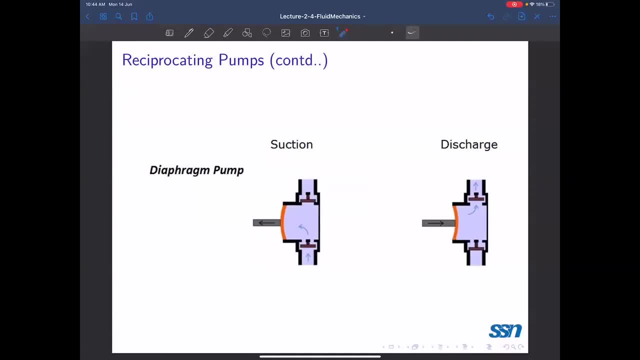 the energy to overcome the fridge. okay, this and all. we'll see in the coming class. possibly we'll need to have some half an hour of time extra time so that we need to have some kind of mock test. also we'll see. okay, with this, we'll finish today's class and let me see how. 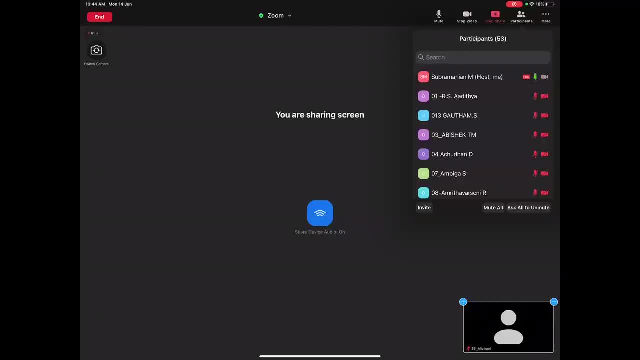 many are available. how many people are there? 53, two people. okay. okay, I need not take attendance. you can go to the next class. you can identify your neighbor and let me know who is not there. number 11 is not there. I'm there, sir 11, so better you name rename. 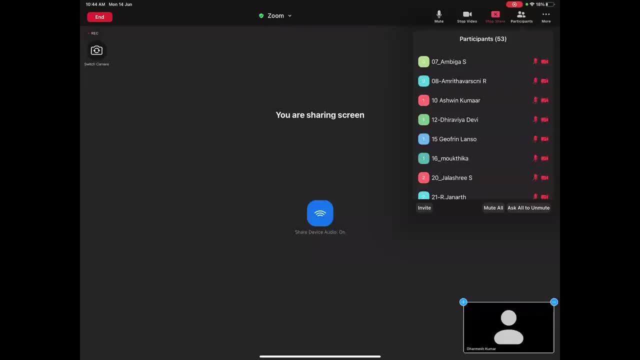 yourself in two sml or two digit register number. it will be easier, so I need not call you people. okay, Dharmesh, you try to rename yourself in the coming class and don't have this three days. okay, Dharmesh, you try to rename yourself in two sml or two digit register number. it will be easier, so I need not call you people. 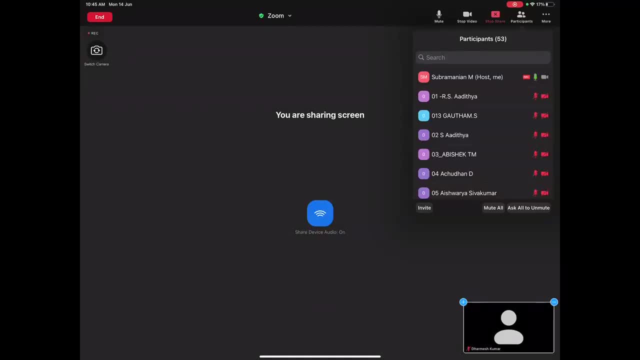 yes, yes, the 가운데, the zero, one three. know, yeah, it's not convenient, and the company and they get us three, one, three. okay, wouldn't it be given for everyone is filled. the next class, I need not. y wonder, will it give you water? not even the next class. I think that I would be able to get a new job. 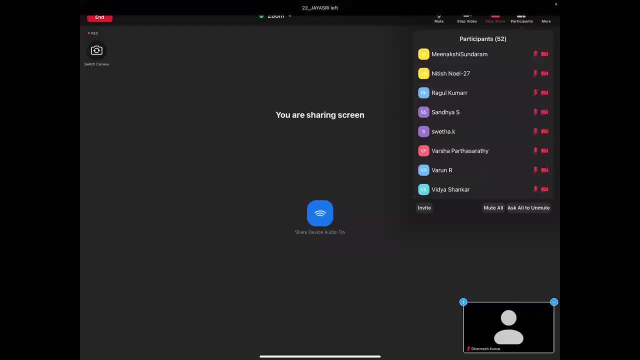 super time. I do time up, so see in the next class. thank you, thank you, sir, but I still have next class back. does this mean? Thank you sir, thank you, thank you sir. thank you sir, is all okay? week start- start of the week available. still, if you have any doubt, you are welcome to. 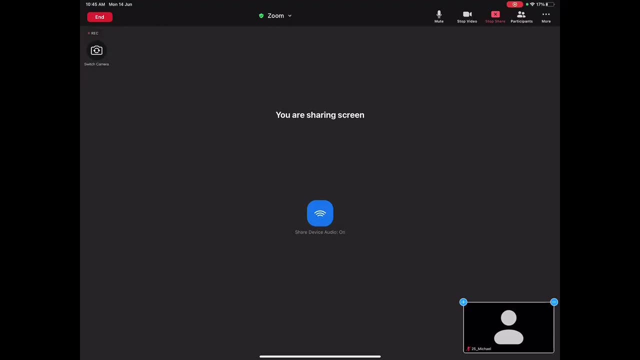 ask because you have another 15 minutes before the next class. Since there is no query from you people, I am closing now.